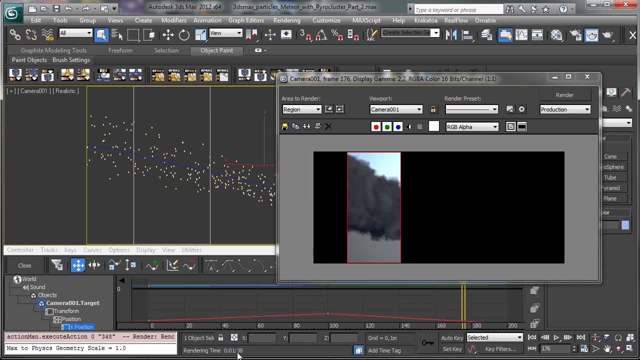 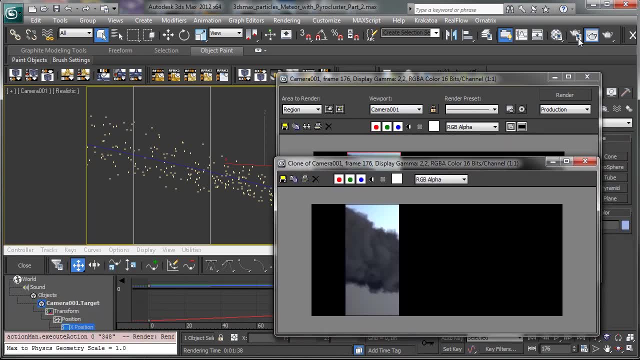 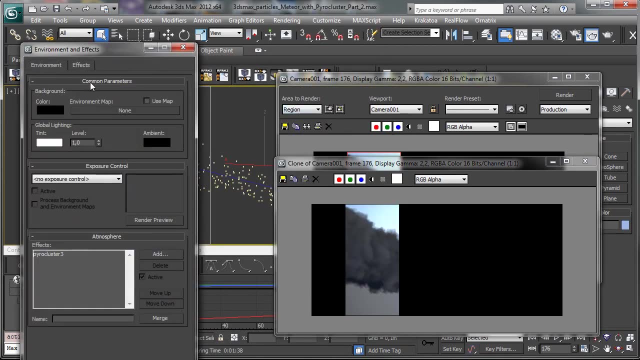 One thing is that I rendered it in 1 minute and near 40 seconds, and that's really really high. We need to speed up the rendering and we can do it going inside Pyrocluster, So we see also how to play with the Pyrocluster parameters. 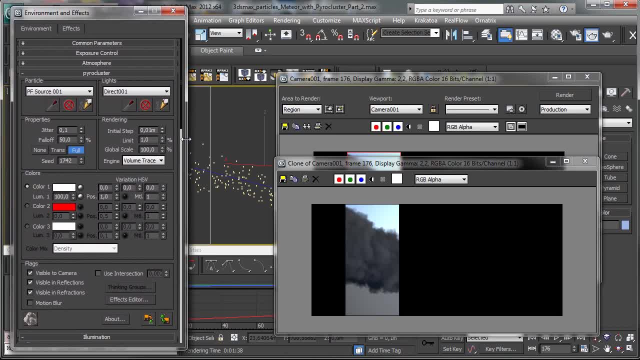 And first of all we can play with the rendering initial step. You see that there we have a sampling quality and actually we are talking about 1 cm. So we can, for example, change and going to 10 cm, because we are talking about a really big smoke. 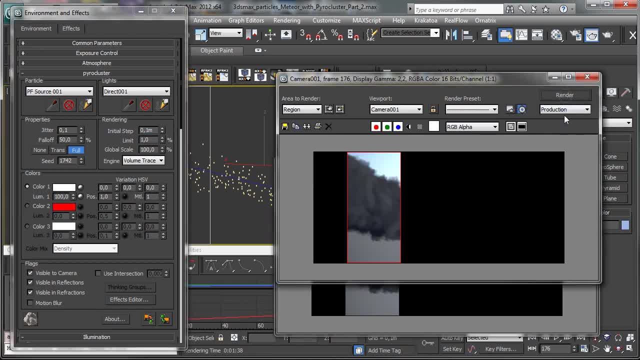 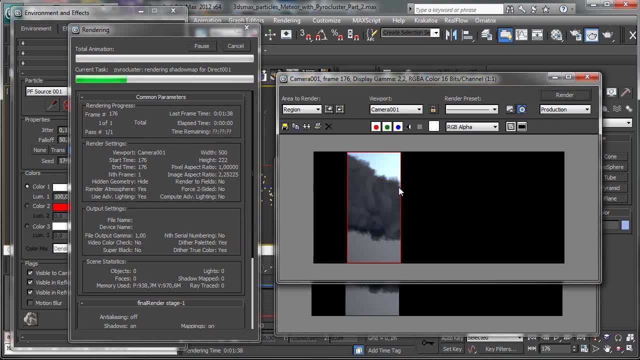 And let's see how it changes in quality. and obviously, if you have to go near the smoke, it is better to have an initial step really low, Because you need a lot of detail. But let's see in this case if it is going ok or not. 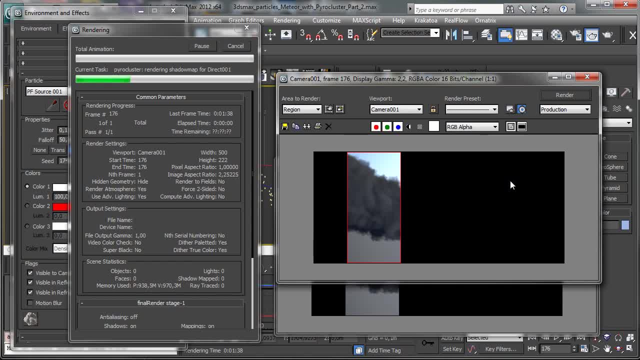 Let's wait. it is rendering the shadow maps, and obviously we have to do the same thing also on the shadows, Because the shadows are really, really slow to be calculated. So let's wait and see to speed up also the other things. Then after the speed up process we have to work a little bit, not just on the smoke area there. 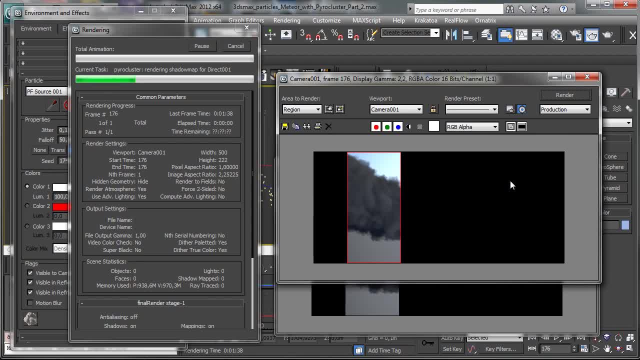 Maybe at the end of the smoke trail and at the beginning of the smoke trail Because I like to work a little bit on the look in rendering and then trying to figure out to obtain a really good quality there And finalize it in compositing. 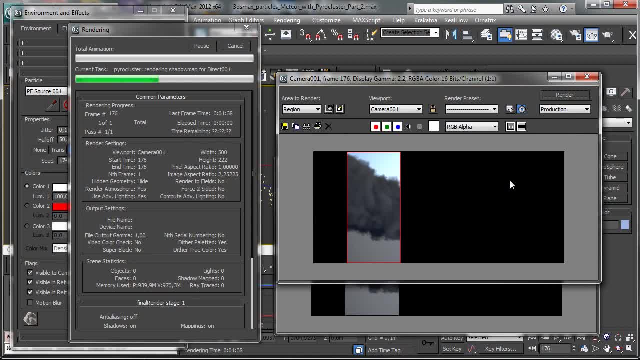 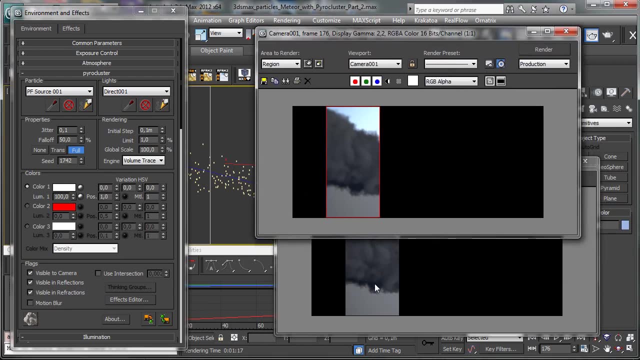 But there we need the right quality to play in comp. Let's wait. Ok, so actually we have 1 minute and 17 seconds and that's something really similar to this one. Maybe we have a little bit less detail. you can see there. 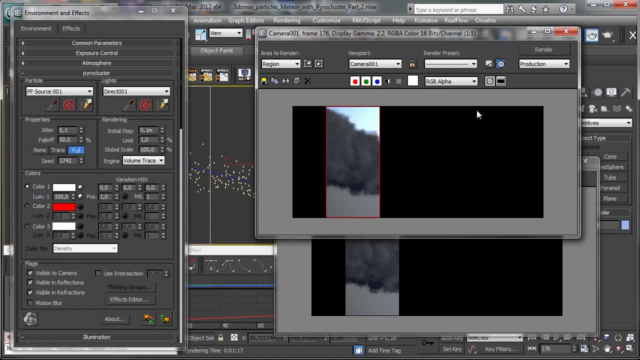 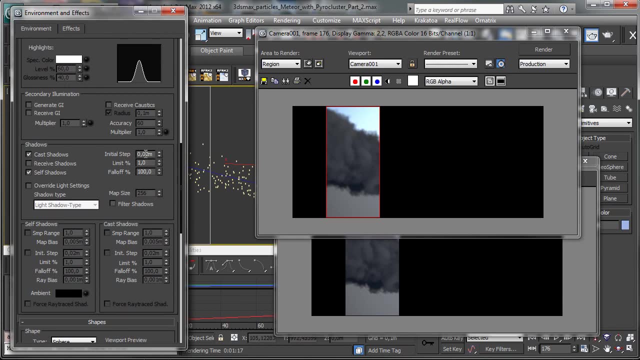 But it is a really fast moving smoke so it is not so important. But it is not so much because we have just 20 seconds less than before. So let's go inside the shadows and you see that there we have the initial steps, set to 2 cm. 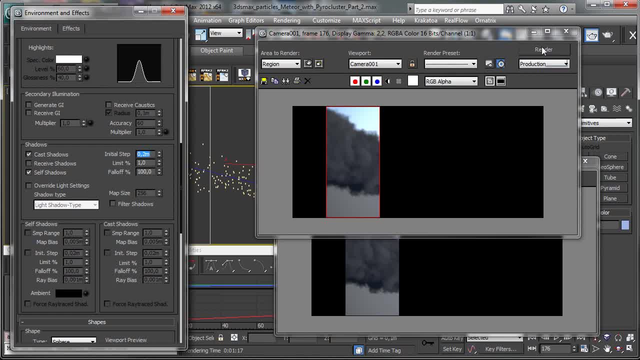 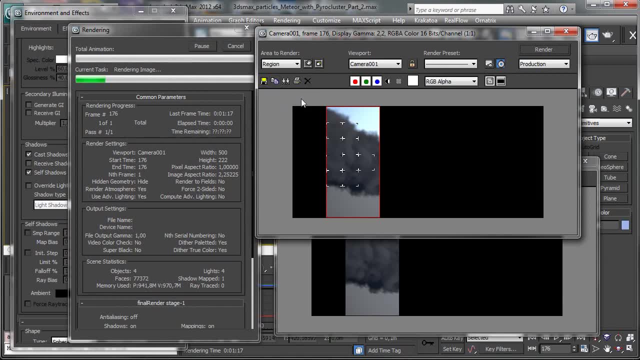 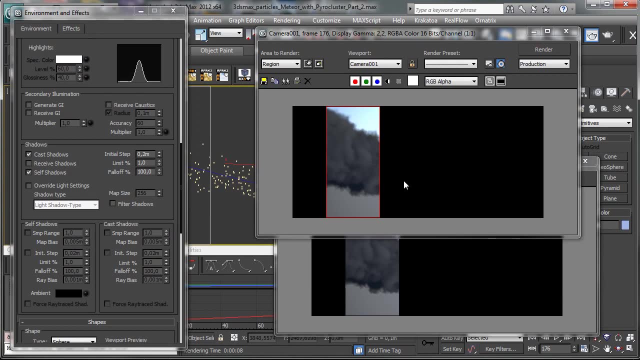 Let's try to go to 20 cm and re-render again, And you see that this time the shadow maps is really fast to be calculated And we have an amazing 8 seconds, So this way gives us the possibility to go back there inside the rendering. 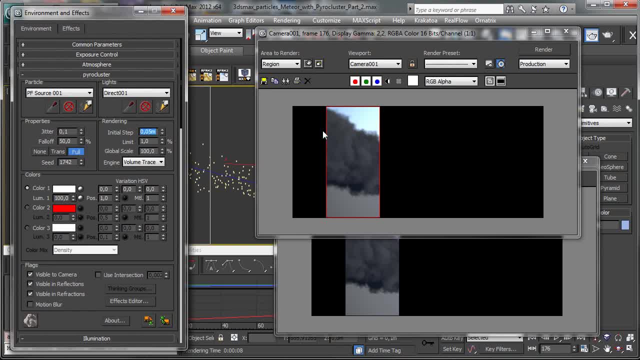 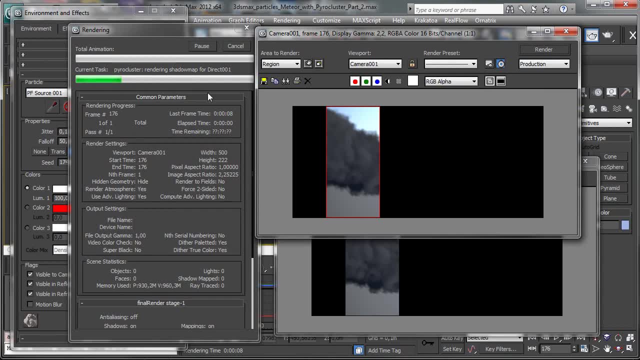 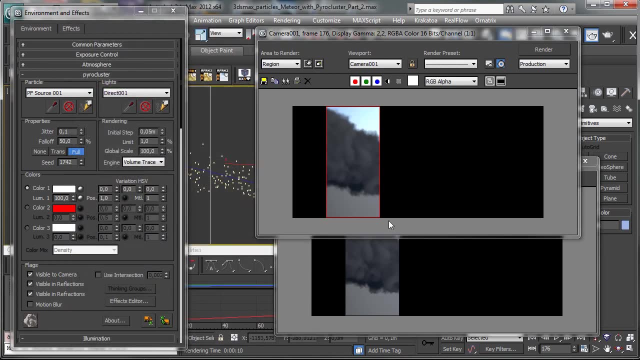 And trying to figure to have an initial step set to 0.05, so 5 cm, So we have more detail. you see that we have obviously a little bit less speed, But we'll have for sure more detail, something in between the really fast one and this one. 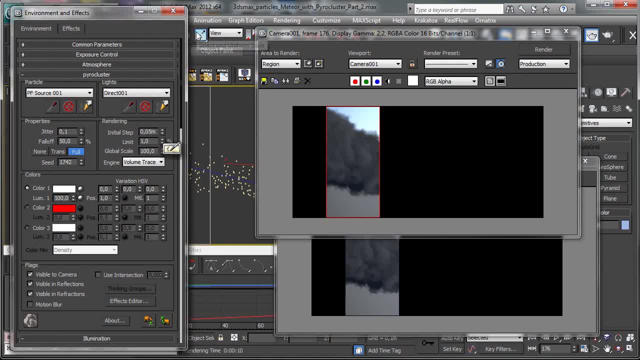 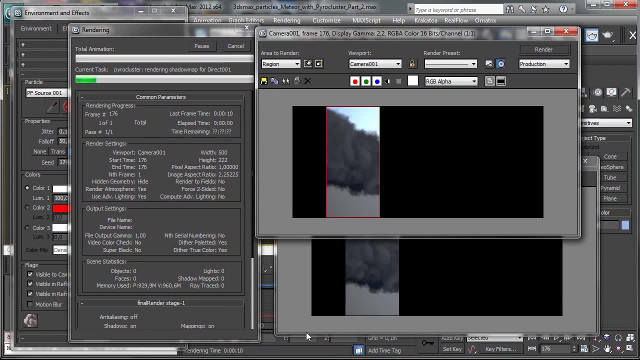 And you see that now we have 10 seconds. Obviously, we can go back to 1 cm and we can see how much it will be slower. We'll have 5 times more detail. Let's wait. You see that we have for sure a slower rendering. 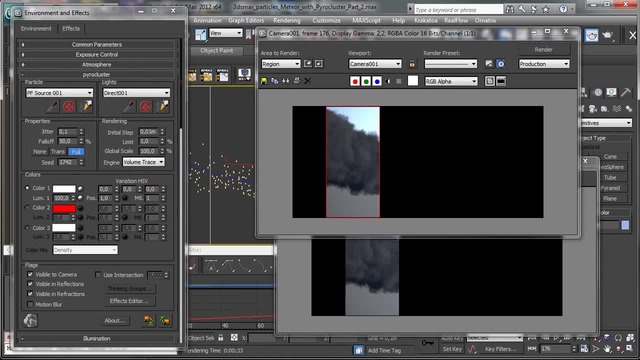 And we have 33 seconds. So we are talking about 3 times slower. So let's think about maybe something in between, like 0.03 for the final rendering, But for the testing we can go for 0.05.. So this was the first step to have a speed up in the rendering. 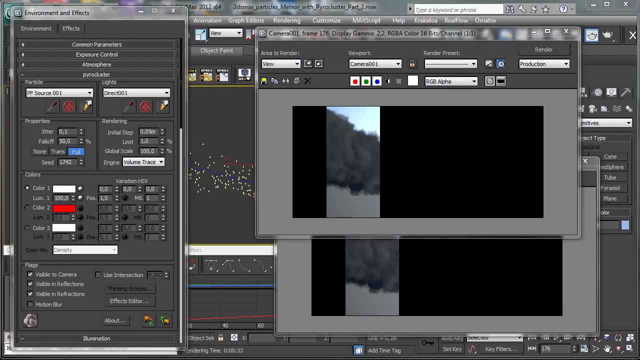 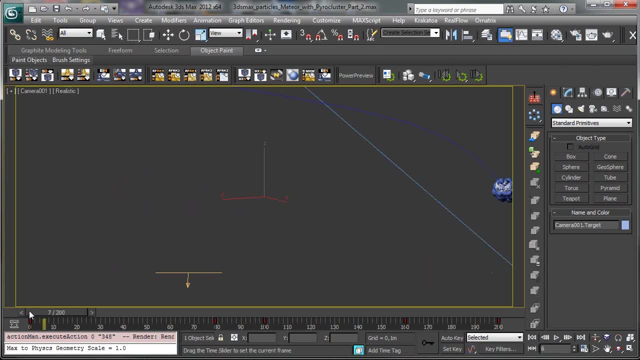 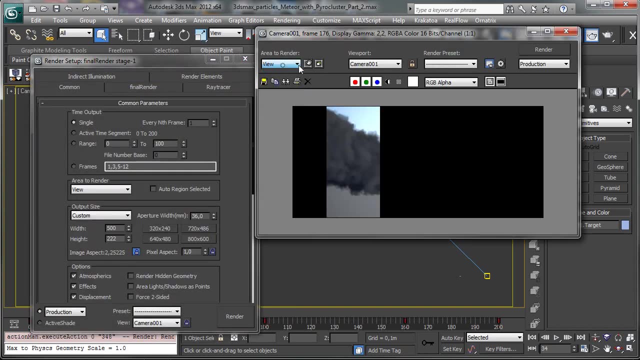 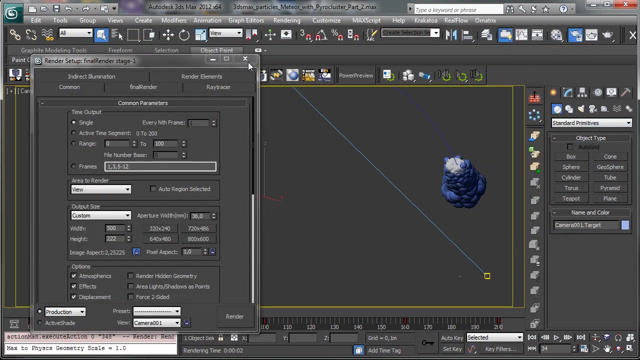 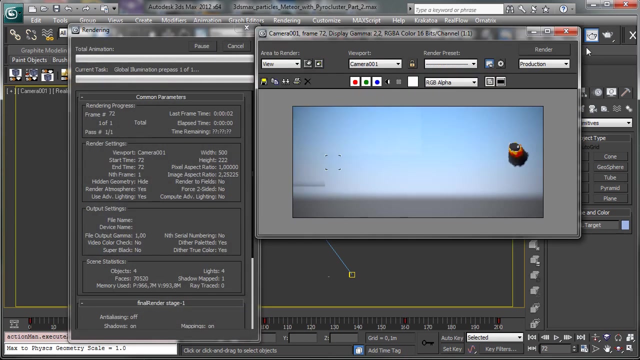 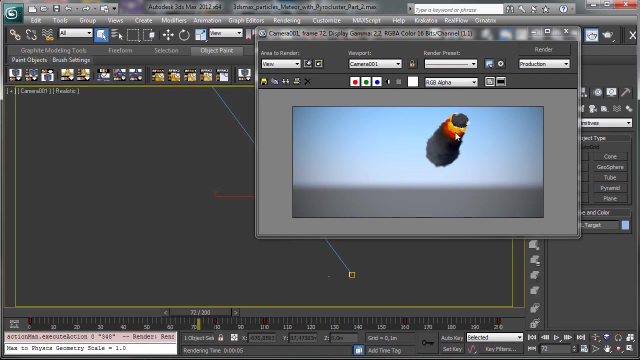 Now I like to check the look on various parts of the animation. So let's see, for example, there at the beginning, Let's remove, ok, and render, And that's what we see there. We have to play a little bit bigger. 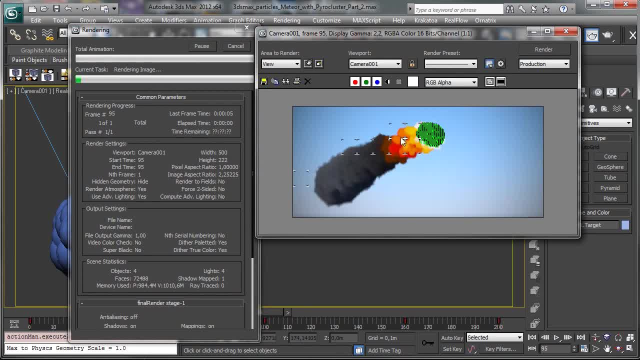 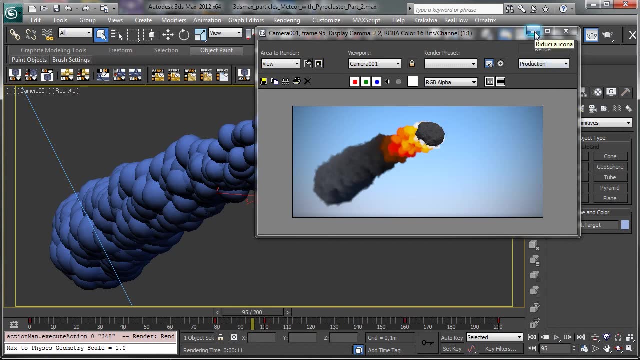 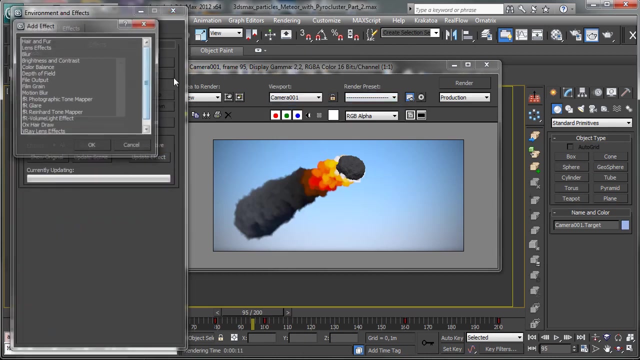 Because, for sure, I think that the quality is not so high, And you see it. So we need, first of all, more particles. It is still, we have still necessity to have a better rendering. I'd like to see, for example, what we can have there. 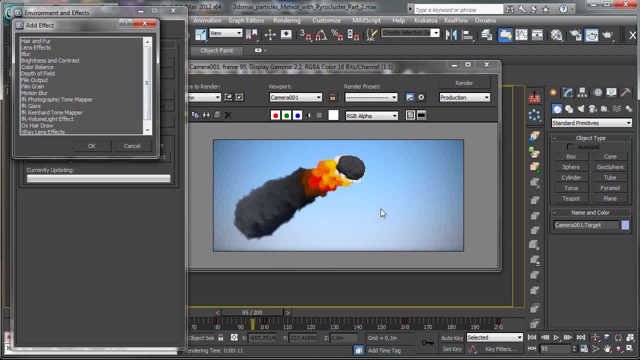 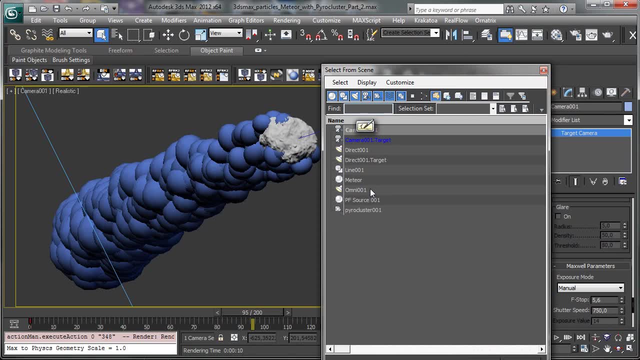 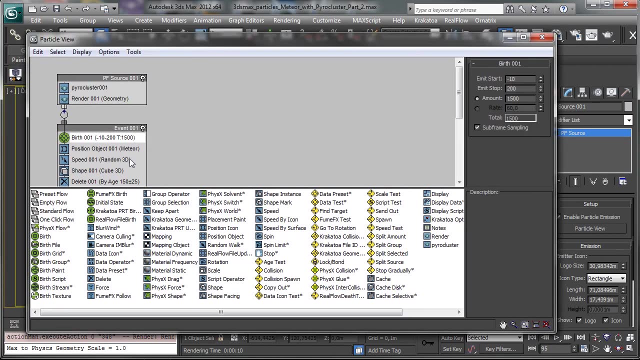 If I use the glow there. So let's start playing a little bit with the, With the particle system, to have more particles at the beginning Let's say that we have, Let's see how much particles we are using. Ok, Let's say we have 3,, 2 times particles. 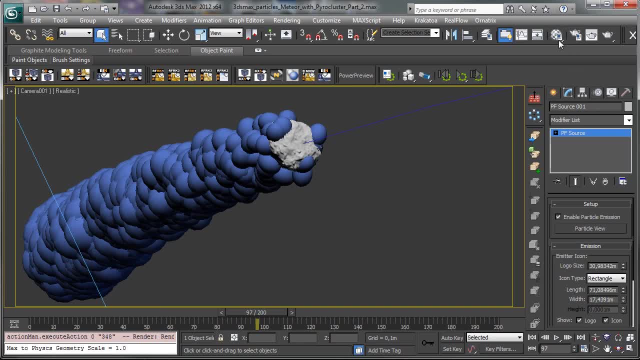 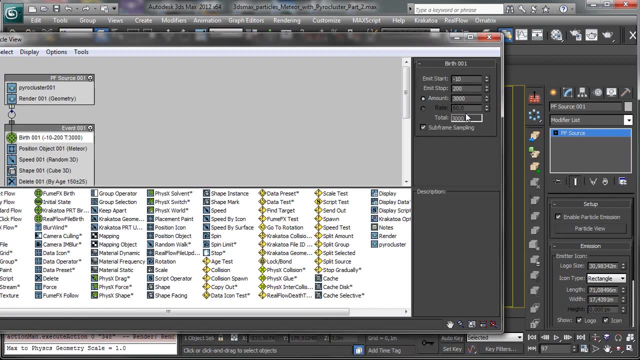 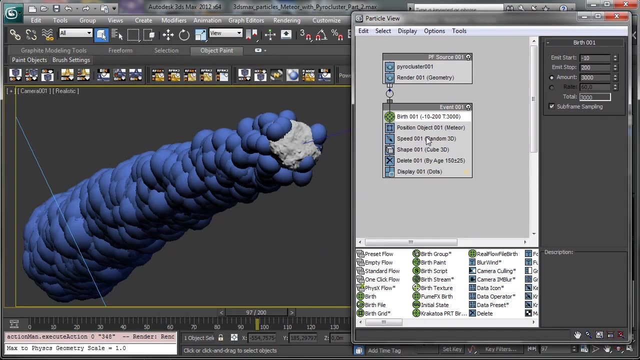 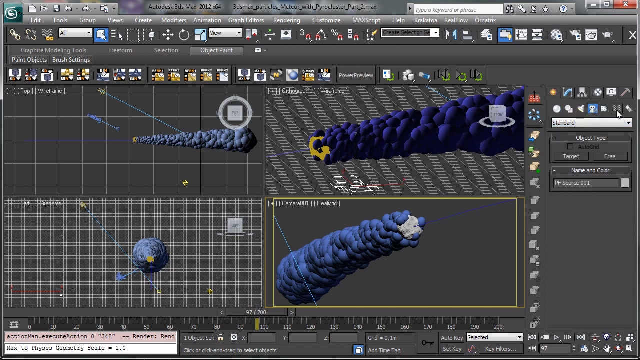 Ok, And let's try to have also A little bit of speed up. We have just a random speed, See without from a speed. Ok, let's try to have a speed In this way, but also A wind In this way. 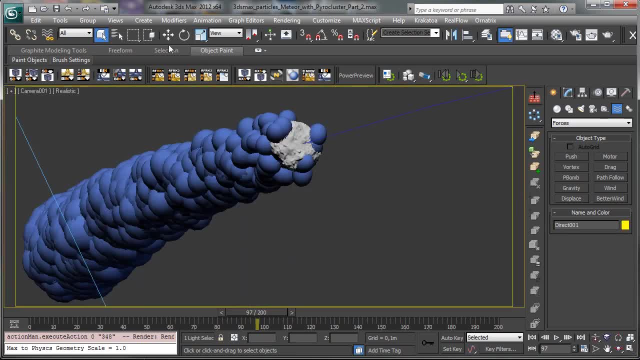 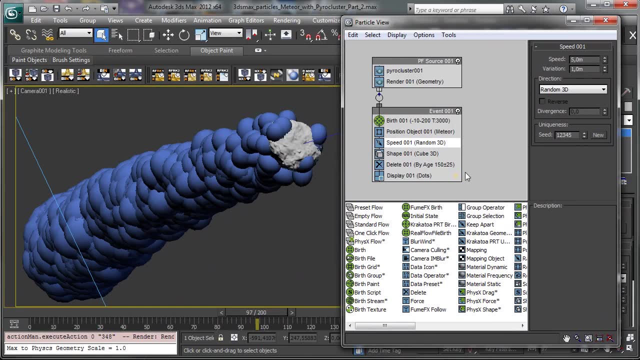 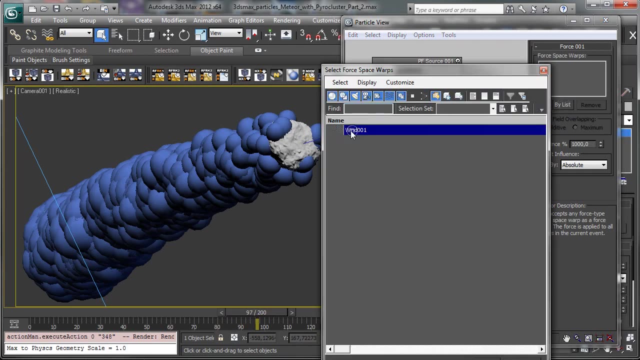 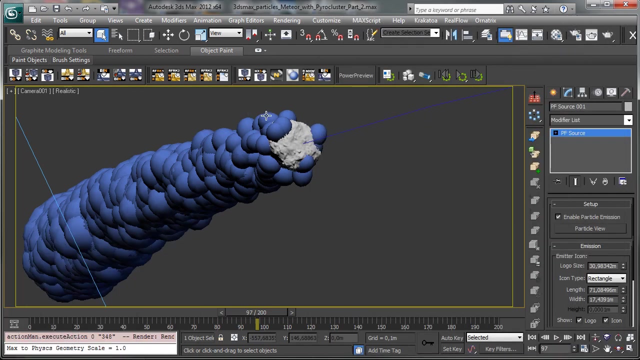 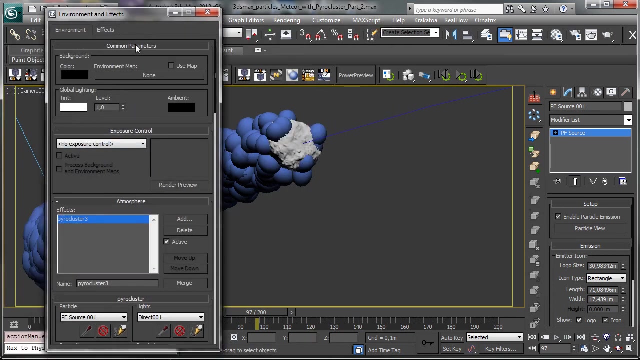 Ok, back in the particles And we can add Another force there By list And we'll use the wind And select Ok. I'd like, just for a moment, to have no Visualization for the pyrocluster, So let's go inside the viewport. 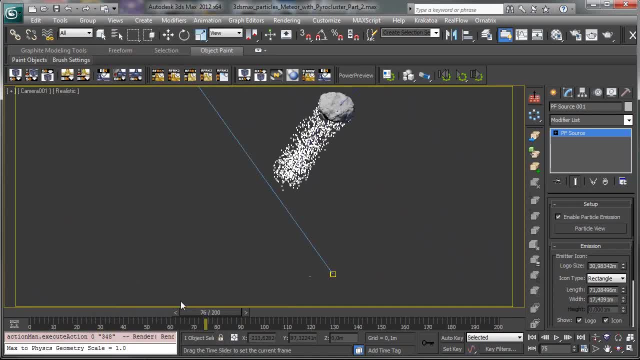 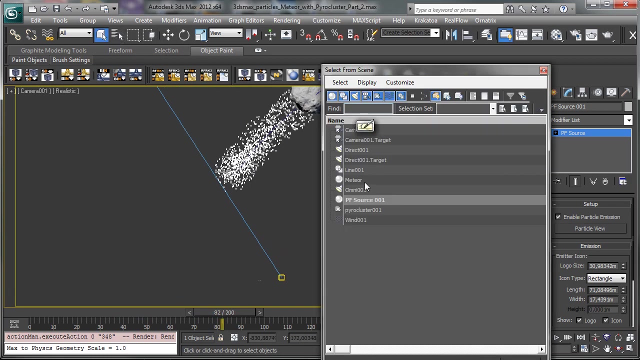 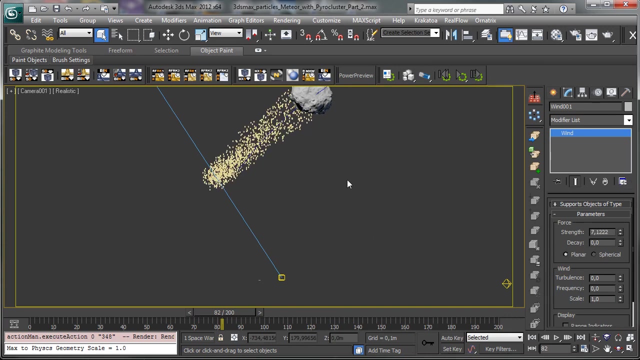 And I say just particles, Ok, Ok. so first of all, We should need To start the animation later, So we have more detail And let's go To the wind. Ok, it works. Ok, And then Let's play a little bit with the speed. 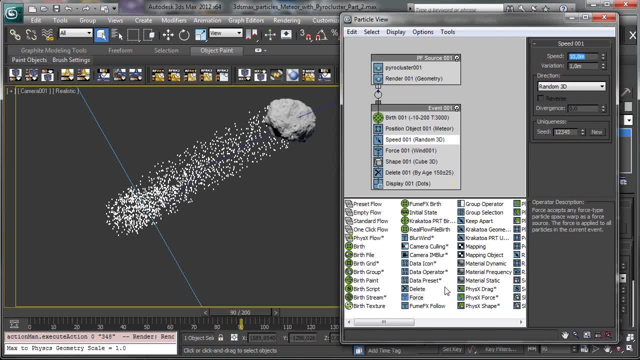 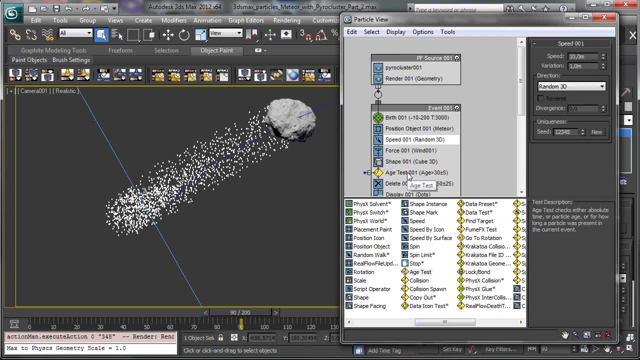 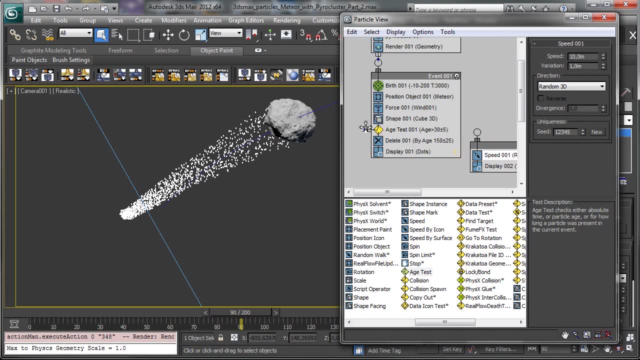 But let's say that the speed is after a while, So we have the force there And then when the Ok, let's play a little bit with the kind of effects We have the speed later When the particles Ok. so 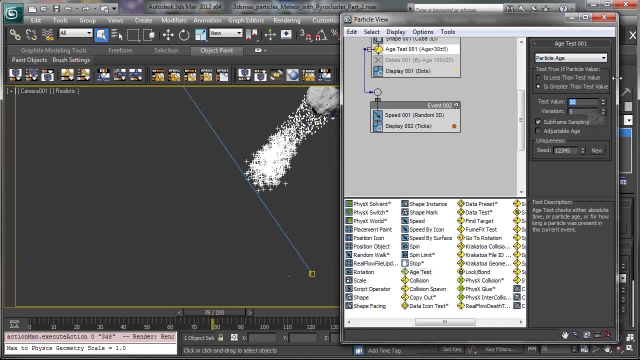 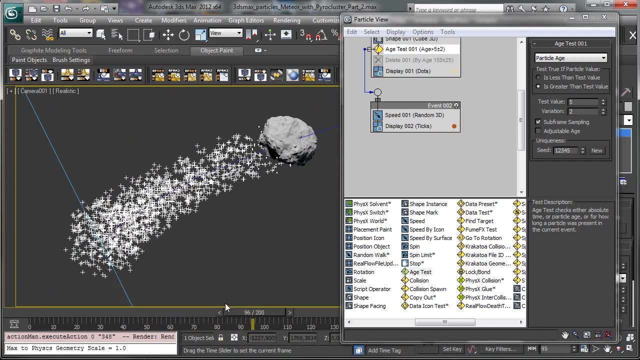 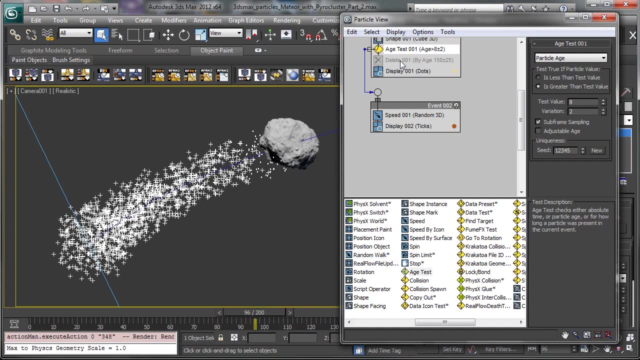 Just a little bit later. So let's say maybe 5 frames And then We have just A speedup At the beginning. Let's try it with 5000.. So we have A really high Force at the beginning. 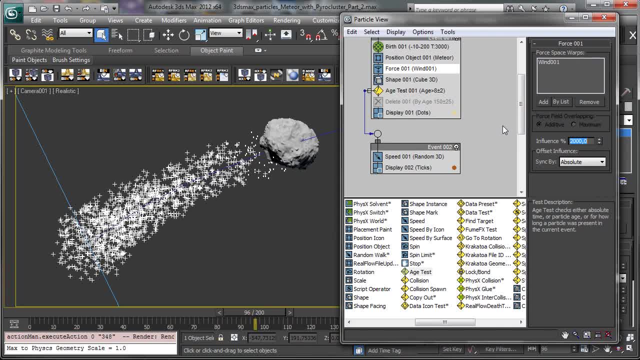 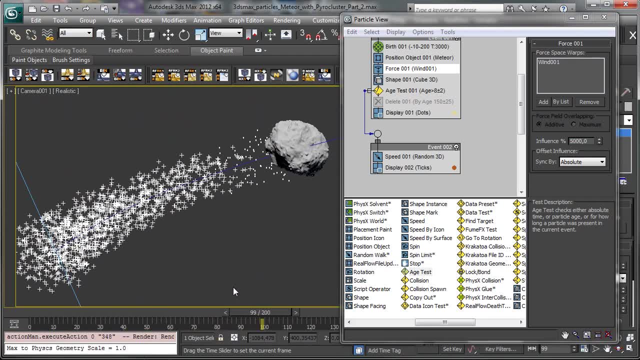 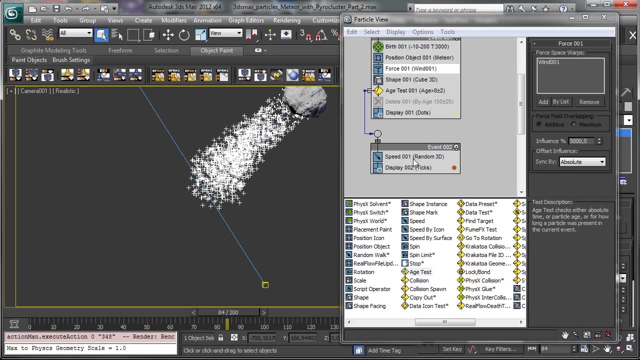 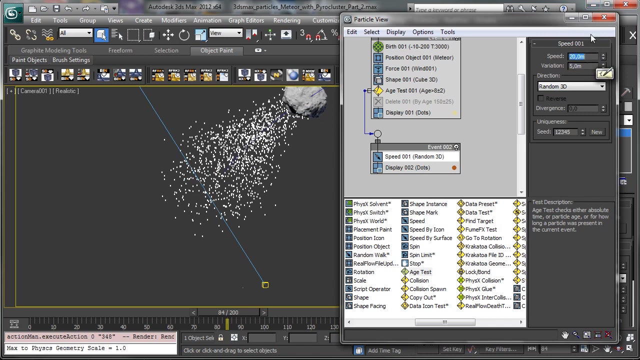 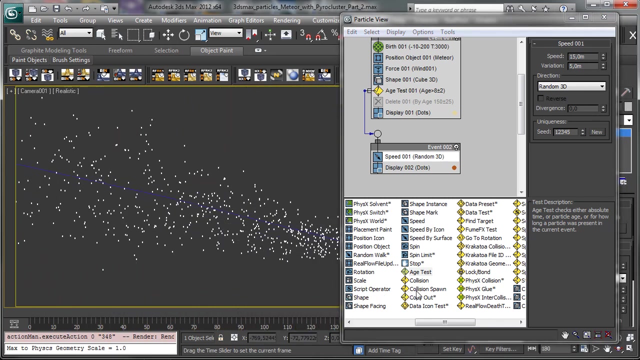 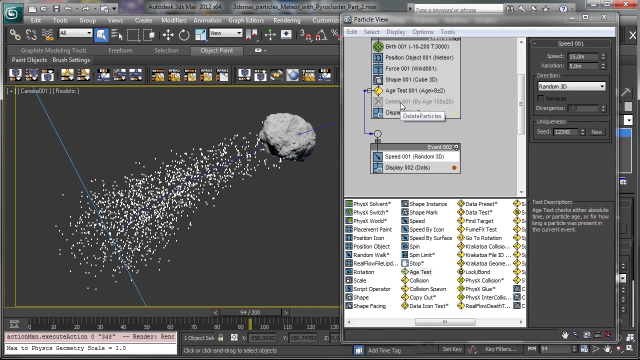 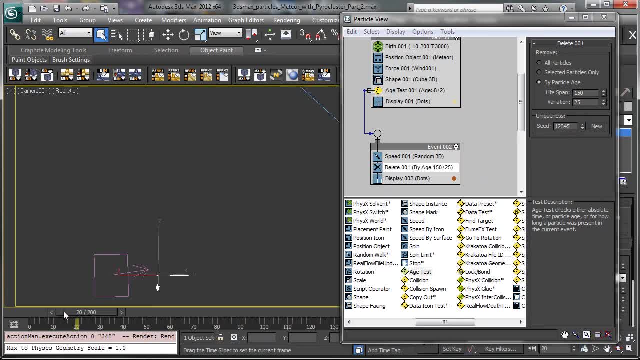 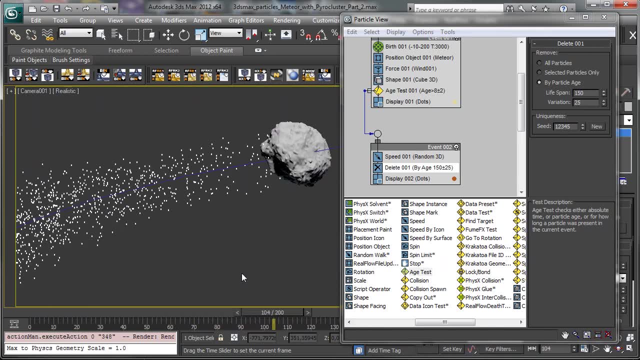 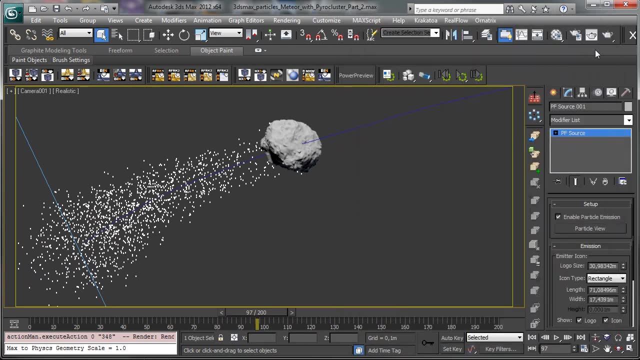 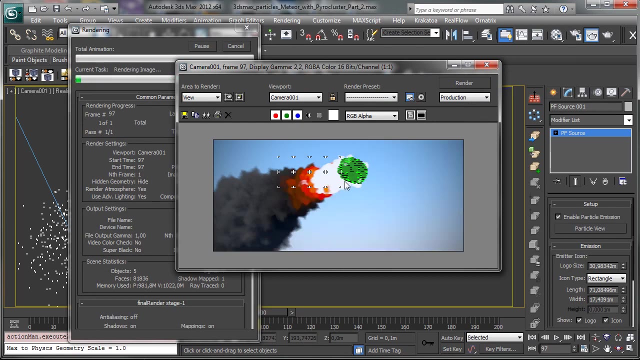 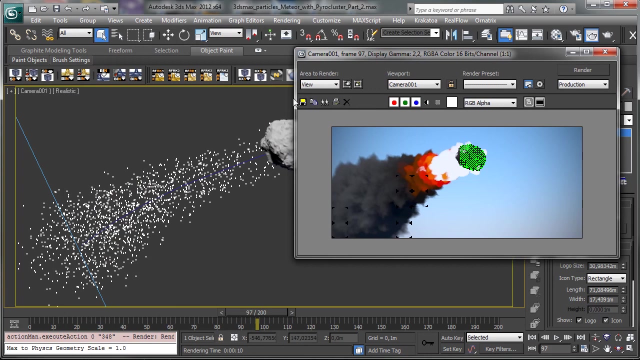 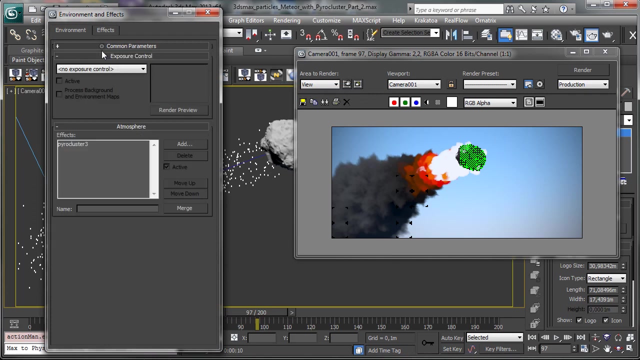 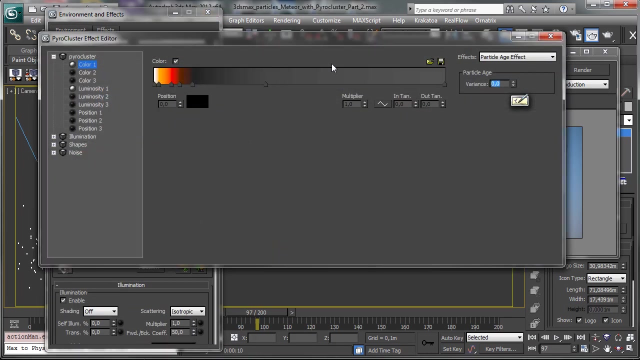 and now it is set to on, so the particles will die after a while. okay, let's see. obviously now we have to play a little bit with the parameters there and also with the scale, because we have to scale the particles later. so let's go there inside pyrocluster, let's work on the color, so we need for sure. 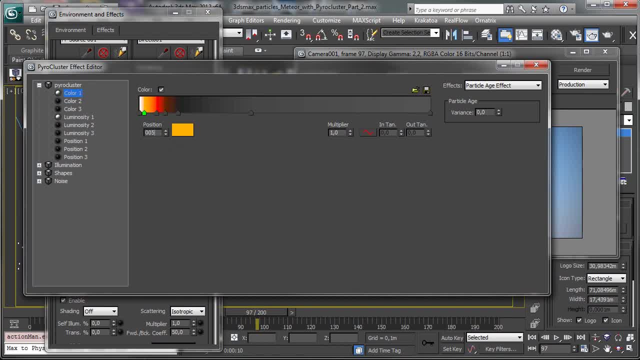 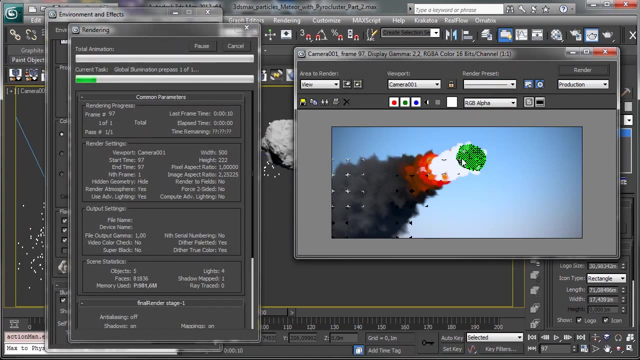 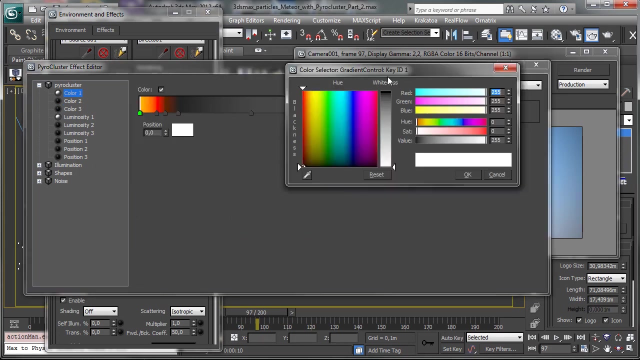 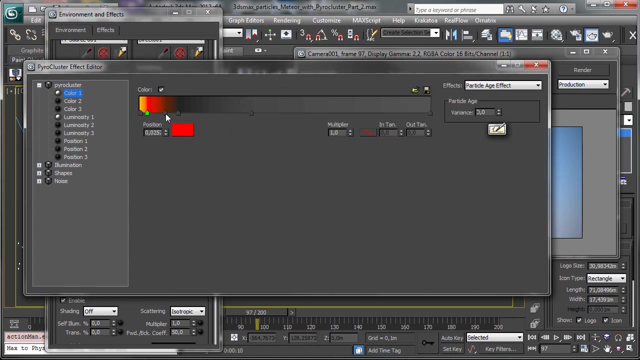 this one set to 0.5, okay, and the other stuffs can remain the same way. we should add white particles just here, but it is still too much present, so we can remove the white color and we'll use another yellow color and then the red, so all the colors are near. 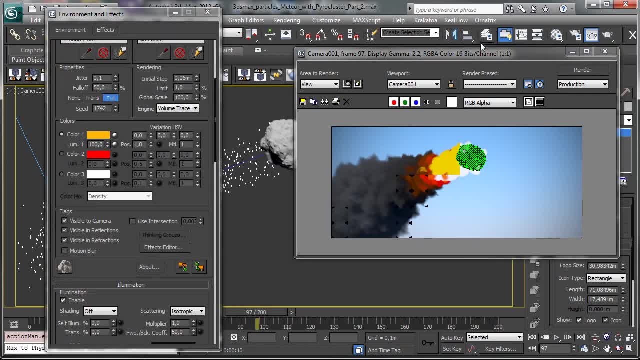 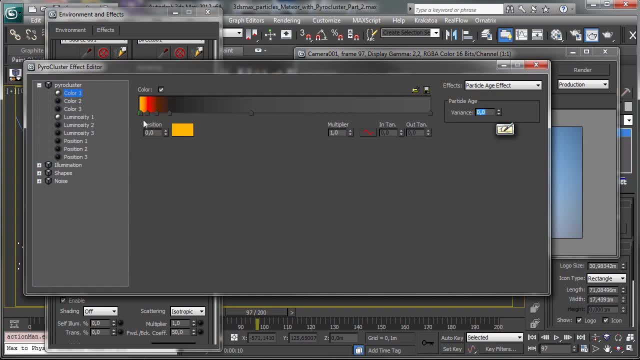 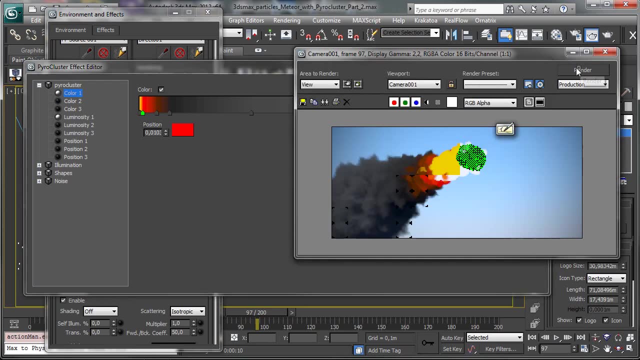 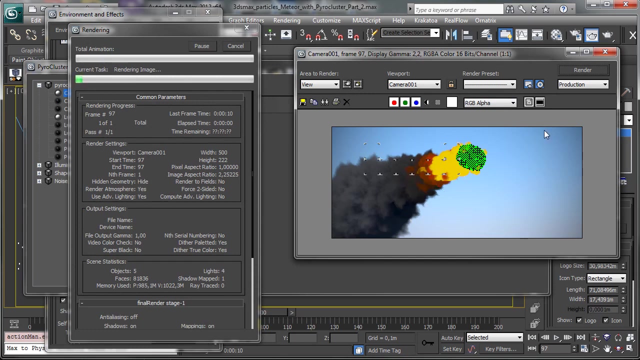 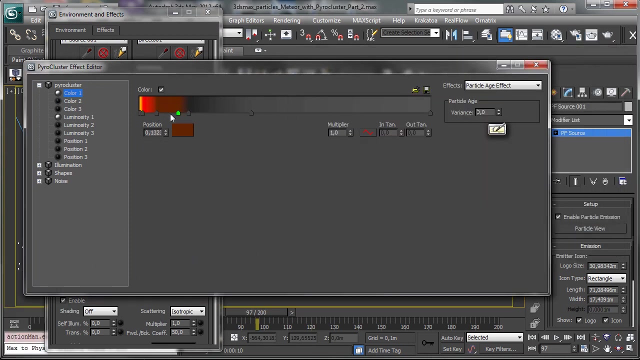 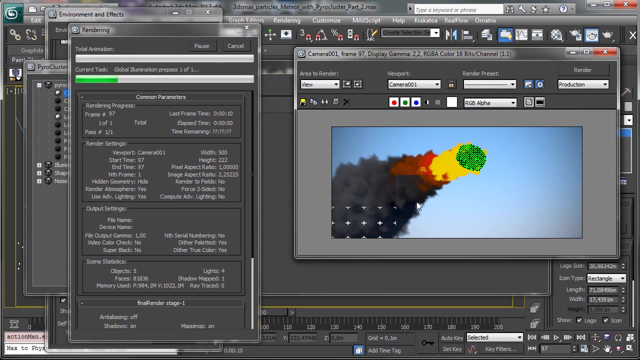 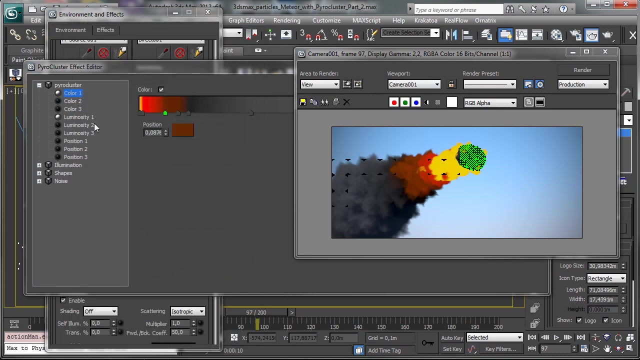 more than before. so the yellow is really big, obviously because? so let's remove the second one and render. we should have a little bit less yellow. it's not so simple because we are using, so let's try to have just more red for more time. okay, let's change the color. 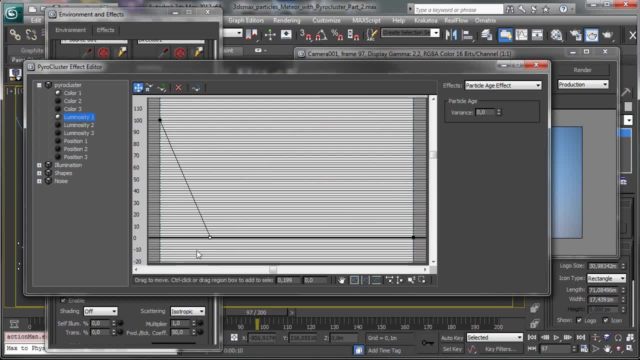 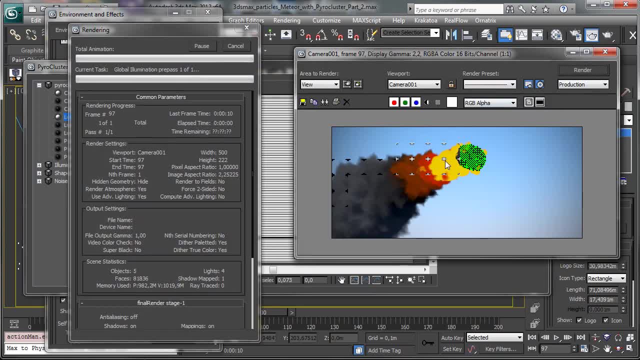 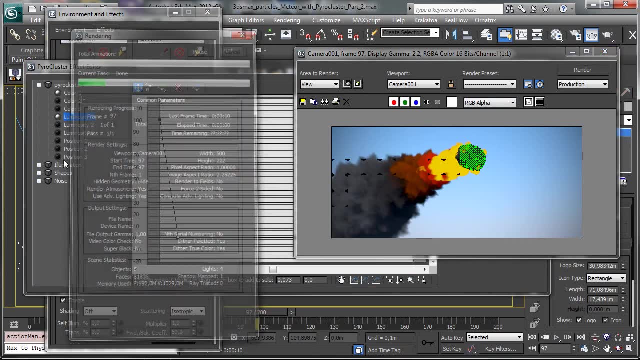 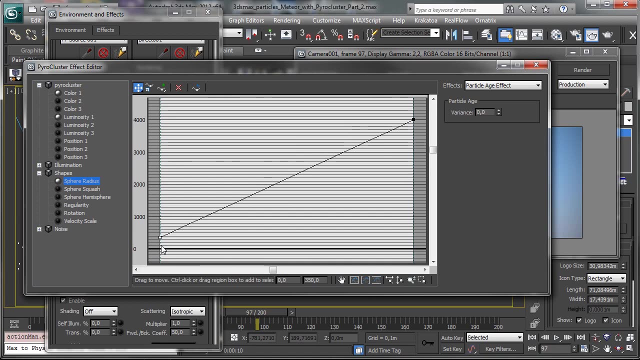 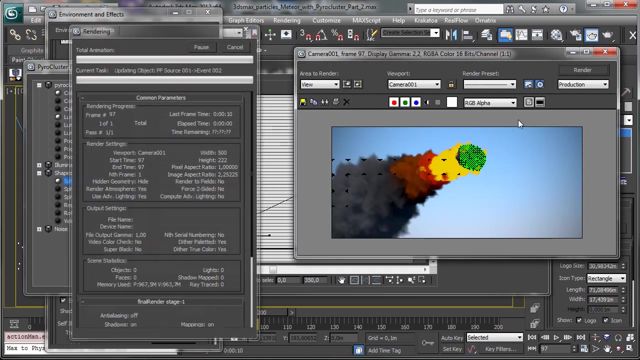 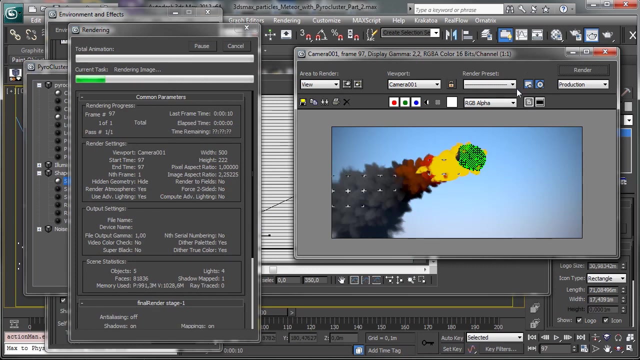 check the scaling and also the luminosity. so this one let's remove. let's see how it looks. sure, we have self illumination, just on the first part. okay, then let's go to sphere radius- we should have. let's see a corner. okay, so we have less scaling. you see, it is slower the scaling. 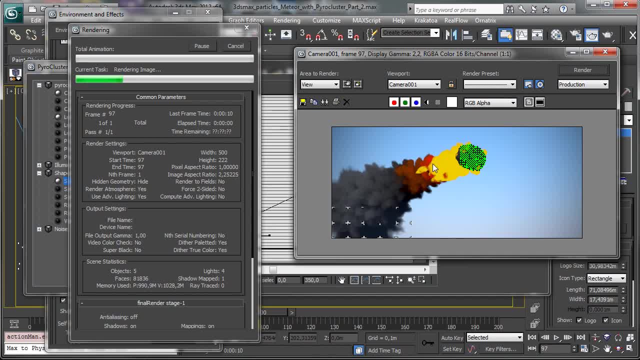 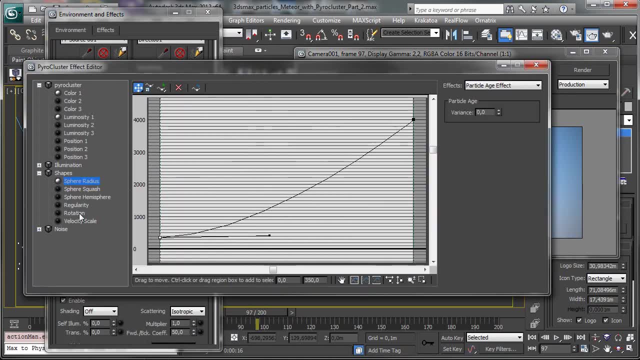 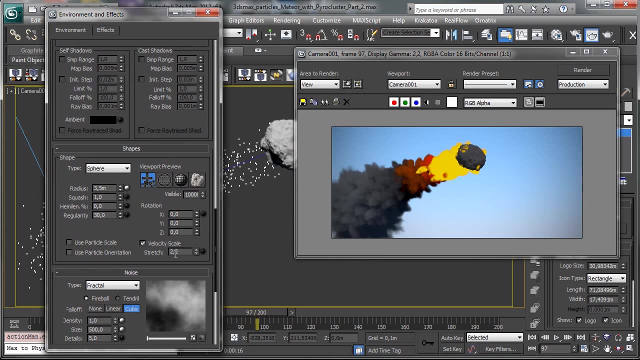 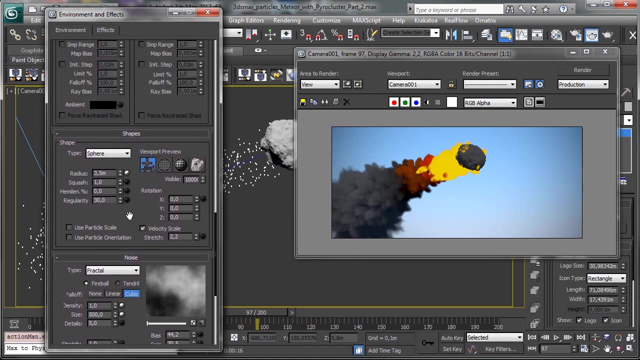 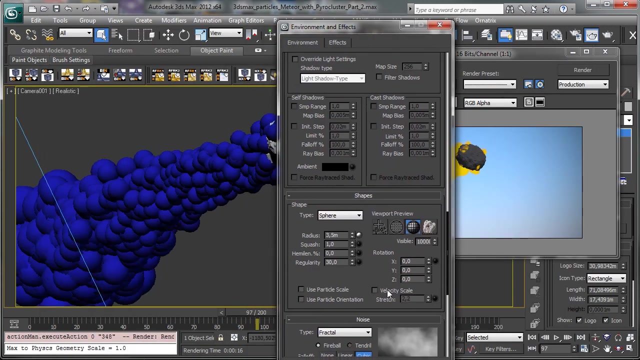 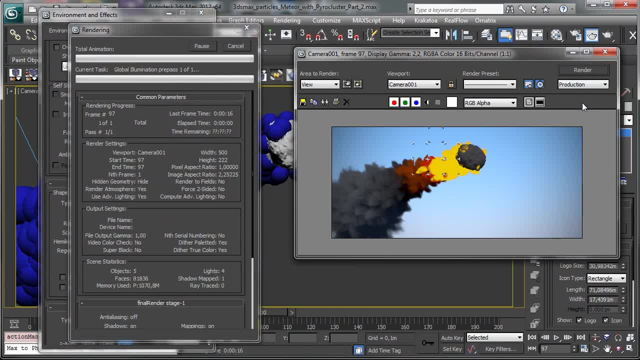 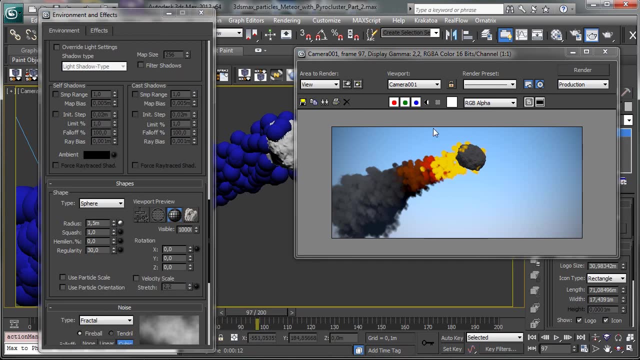 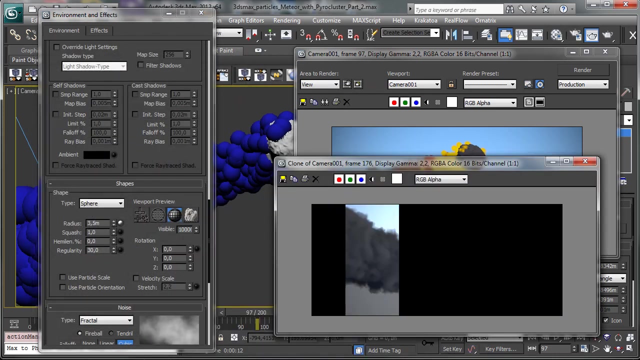 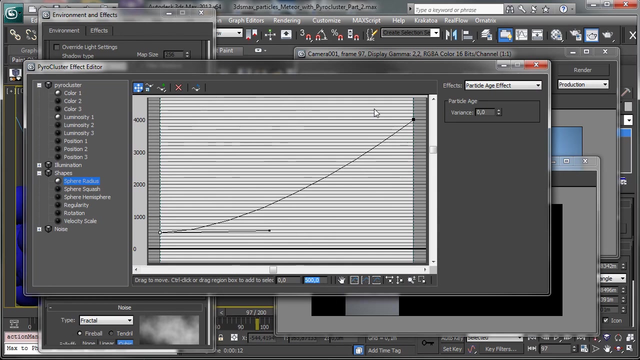 the speed is also in the other, in the other direction. okay, we are back to have a smoke effects, okay, okay, okay, okay, and we need to see bigger particles at the beginning. so back inside the environment. this one is not right one. this one is not right one. okay, there, the sphere radius at the beginning. let's go for 500 and let's see how it looks. 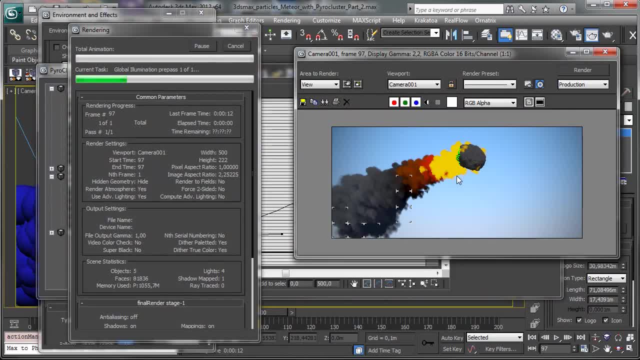 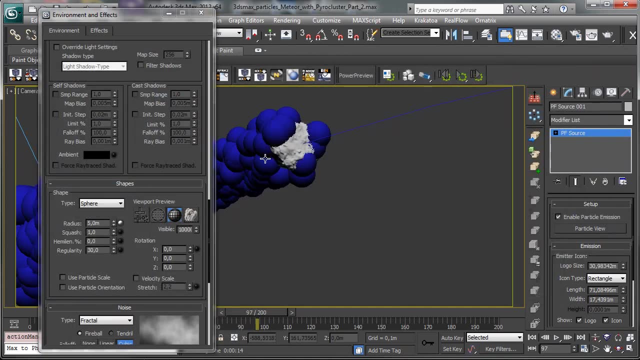 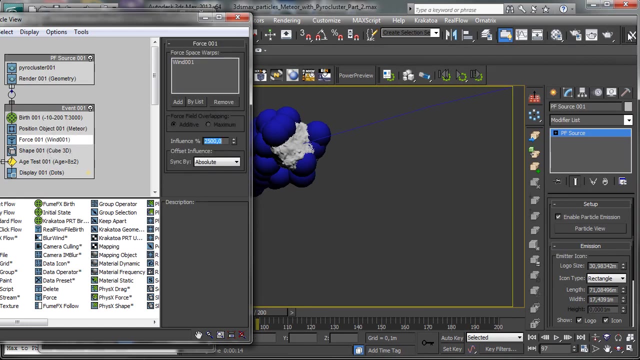 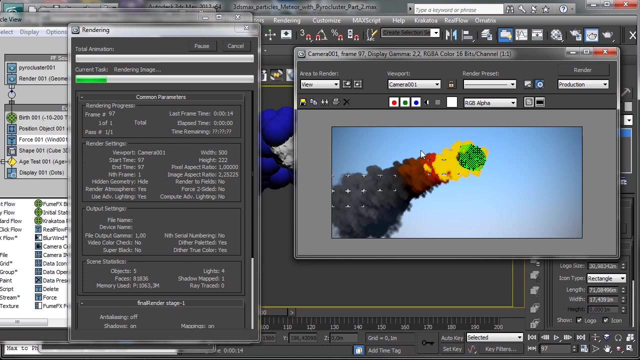 how it looks and we can have a little bit less wind speed there. let's try with 2500, maybe still less 1000. obviously I'm changing something that I've done before, but it's just because I need to check how it looks in rendering. 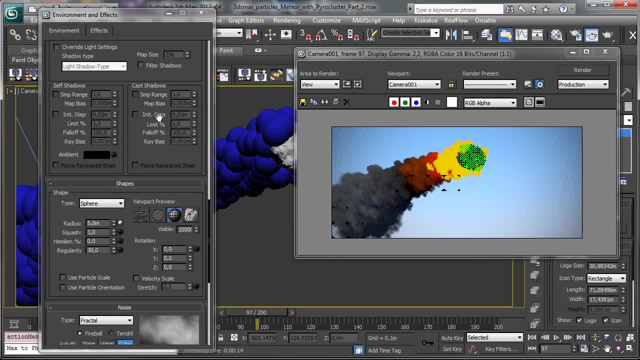 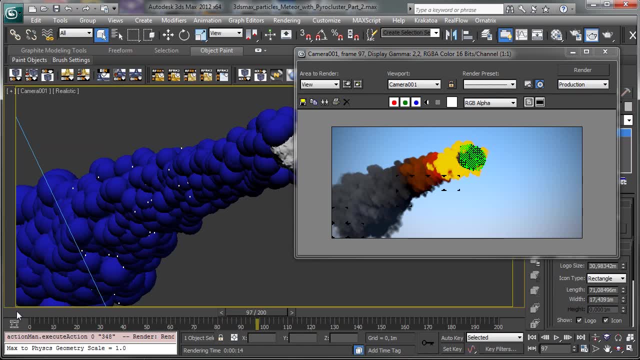 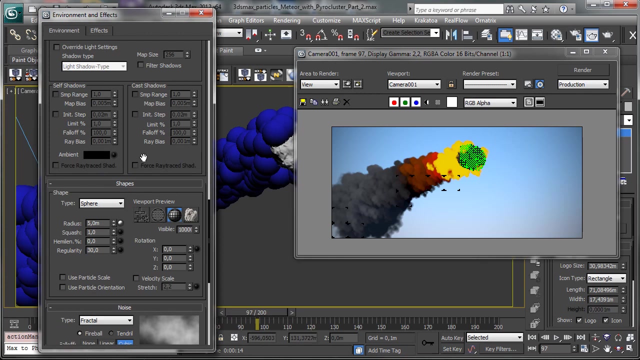 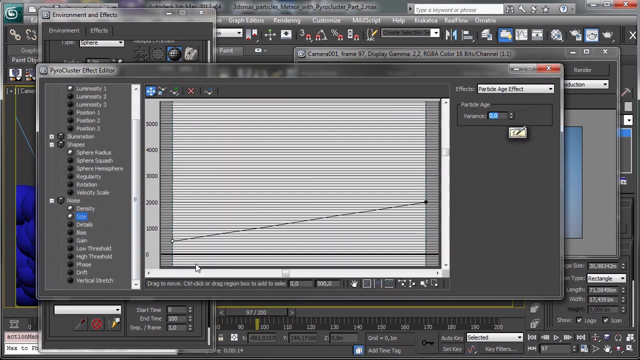 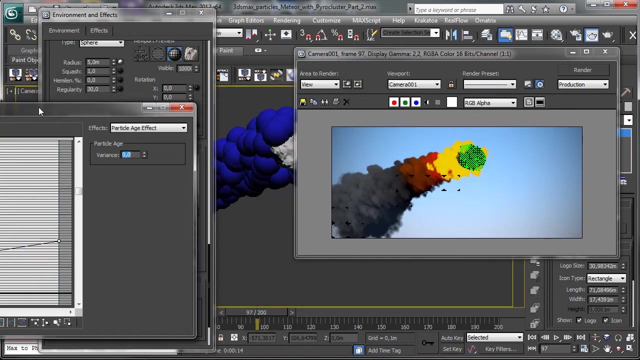 ok, obviously, if you can, it will be better to have the, the asteroid, moving before the camera starts. and another thing: we have to try to scale the look there. so I mean let's go inside the noise sides at the beginning. actually we have 500 and 2000. 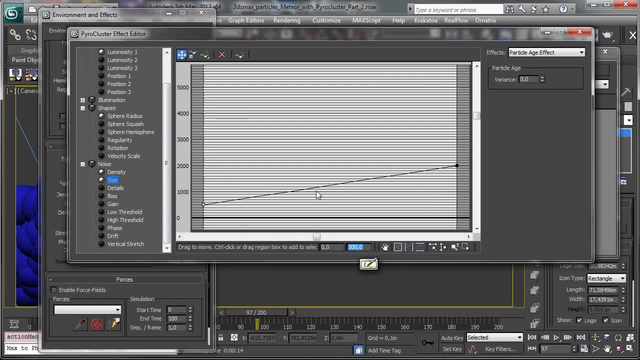 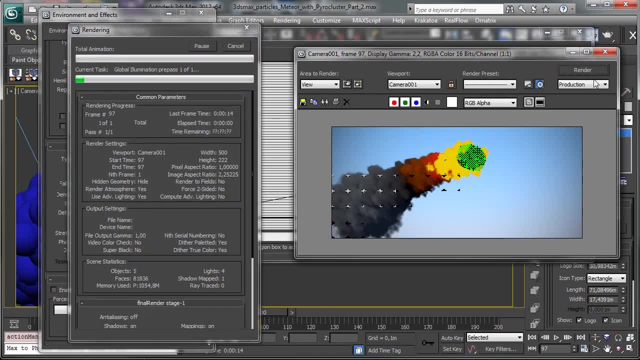 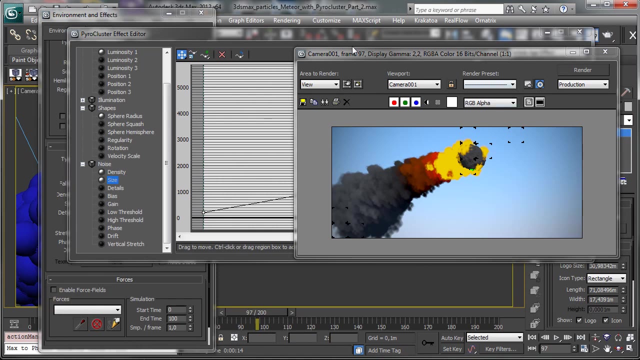 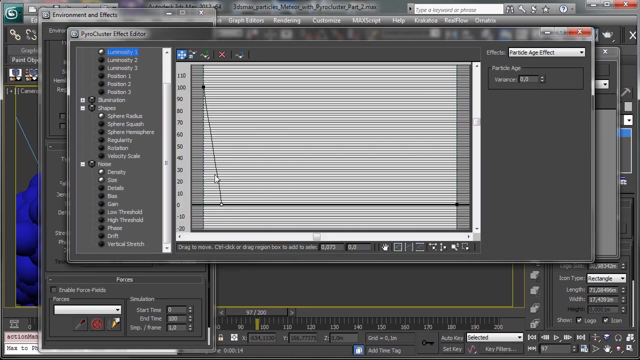 ok, let's try with a really lower amount of detail, and I see more stuff there. Okay, And about the lighting too, again, let's say that we have self-illumination by 75% there, and this one will be 0, but there will be 003.. So really faster we lose the self-illumination, you see. 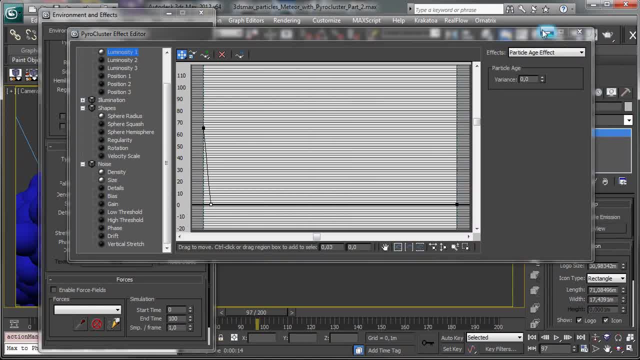 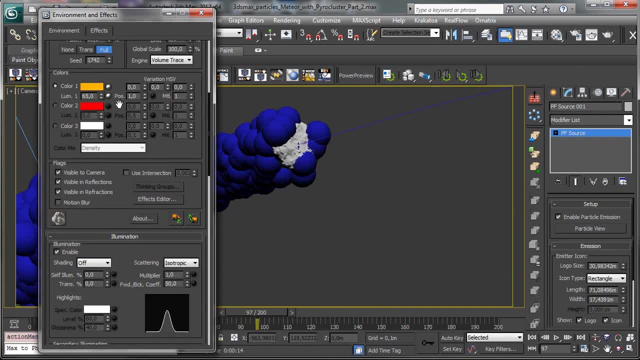 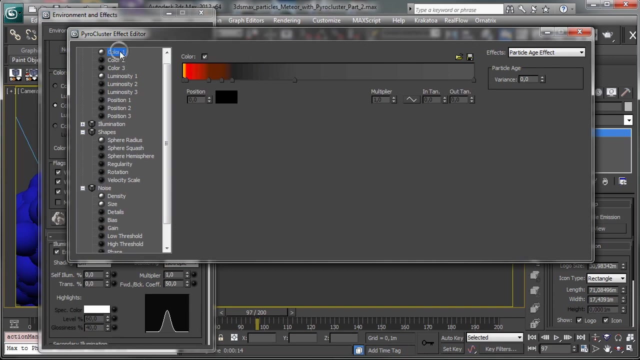 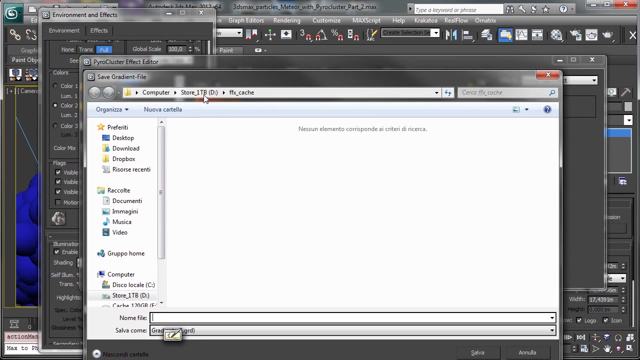 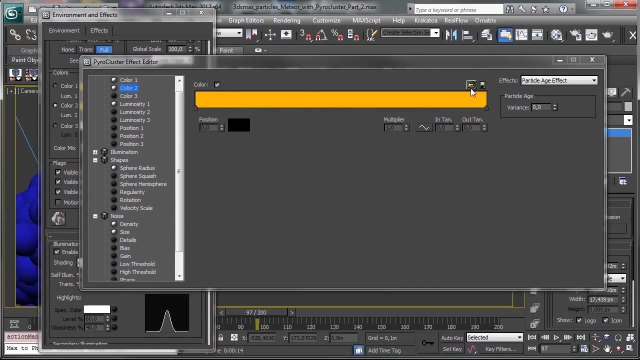 Okay, And I like to have a different color, but it's just a test. Let's save: Okay. there Let's copy and paste. Okay, We have the particle 8. Page effects there And we try to have the same. Okay, So let's save this one And I save it there in a folder And let's call it gradient. There We load the gradient and you see, we have it. 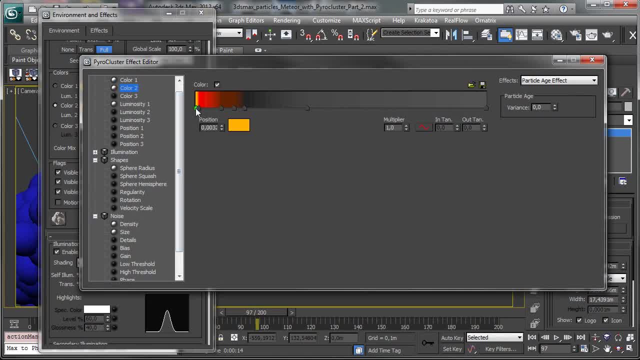 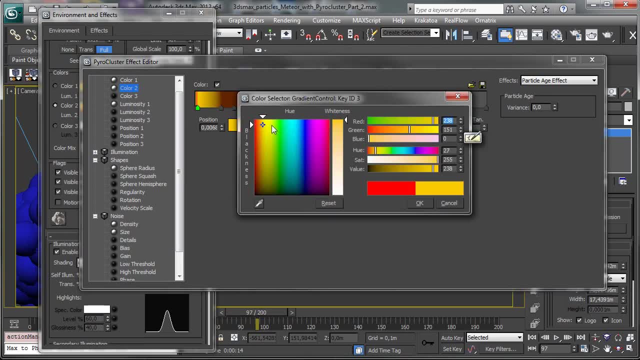 And let's say that there we have Different coloring. So let's say, for example, red, And then there we have the yellow, And then there the red, And that's all, And maybe we can try to have a little bit of dark brown there. 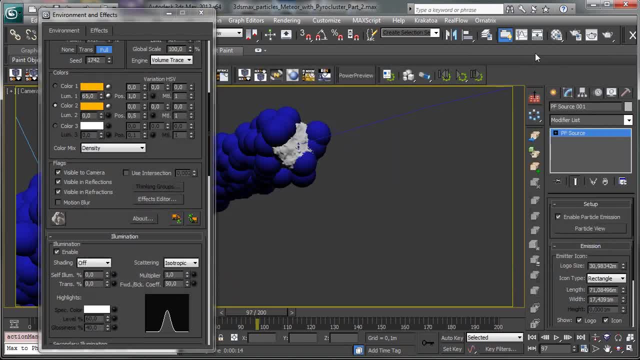 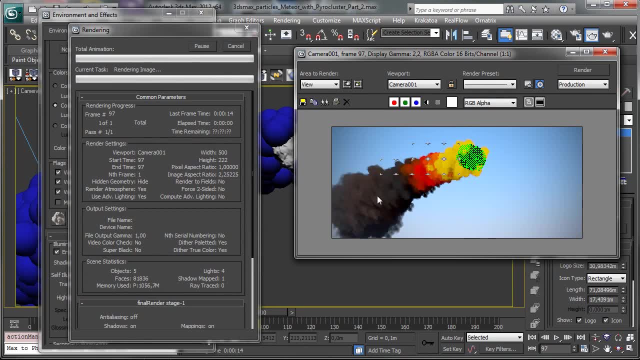 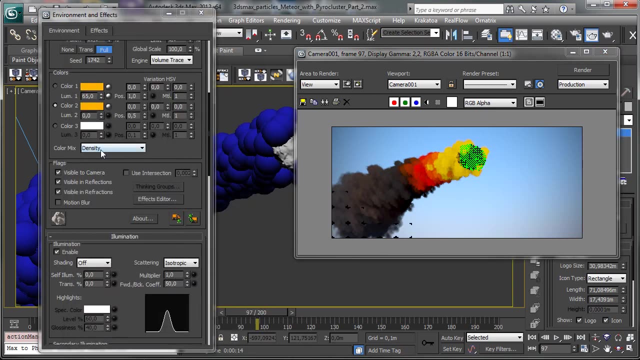 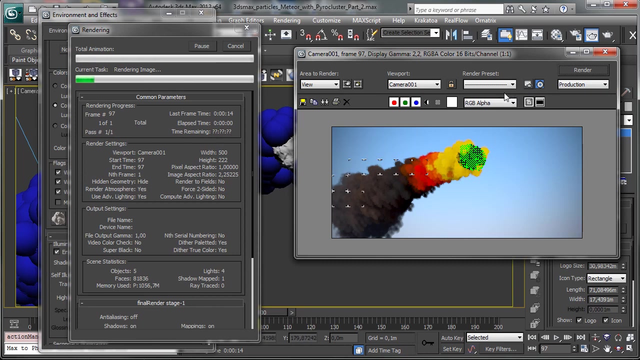 Okay, Just to have some different coloring over it. Okay, And let's see what happened. You see that we have some changes in the coloring. Let's see if we try to use the distance instead the density, We see not so much differences. So let's go back to the density. And I like to have 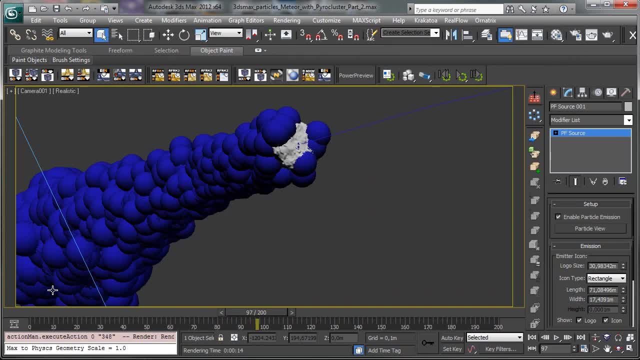 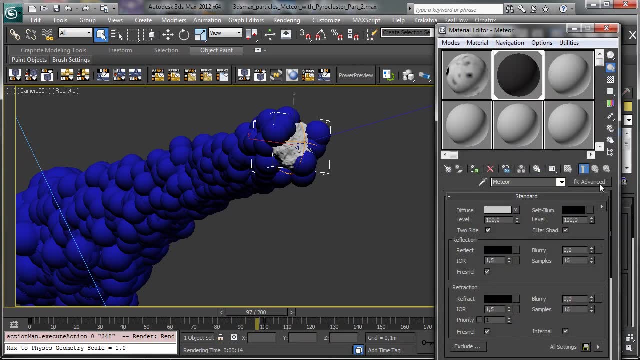 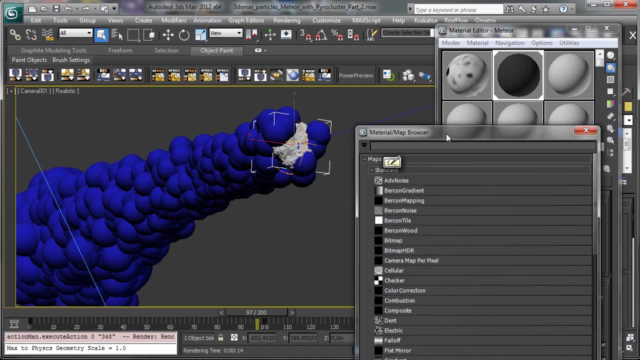 Particles moving in a different way. So let's say that we have a different shader, That's the meteor, And let's see, We have this one And I like to have over it, Let's say, a composite Keypole map. And the second one will be: 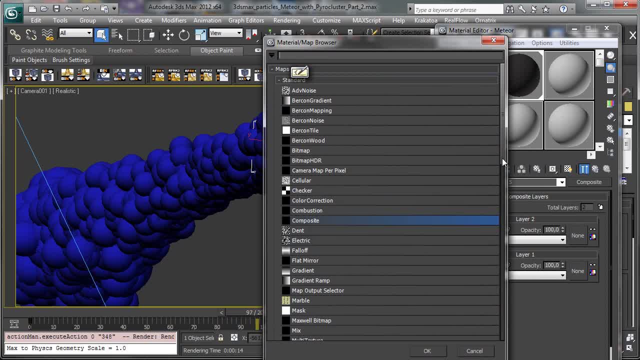 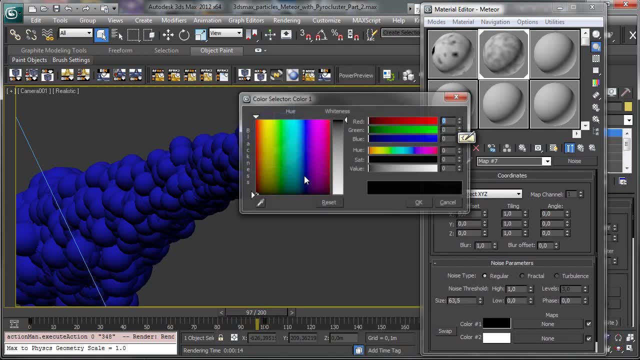 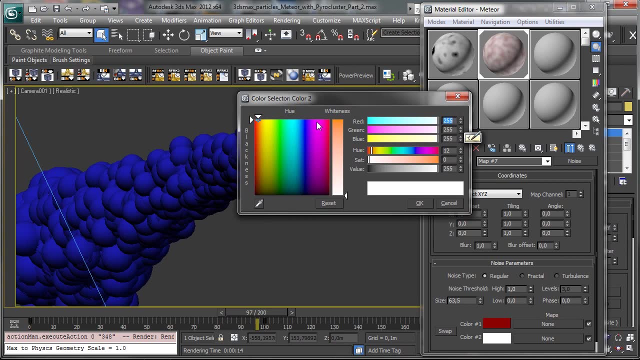 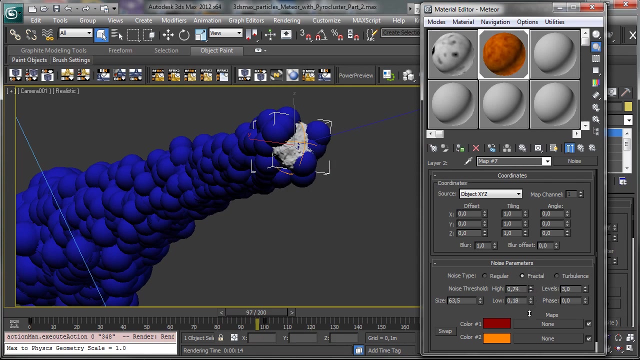 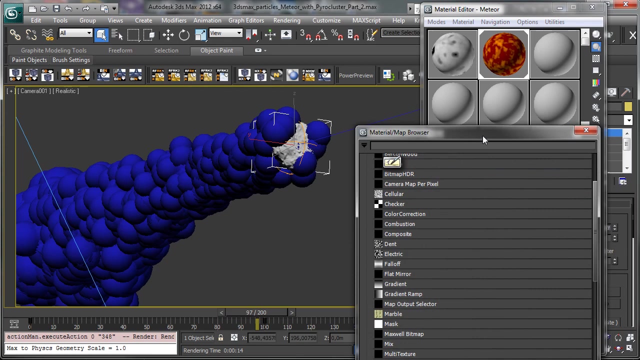 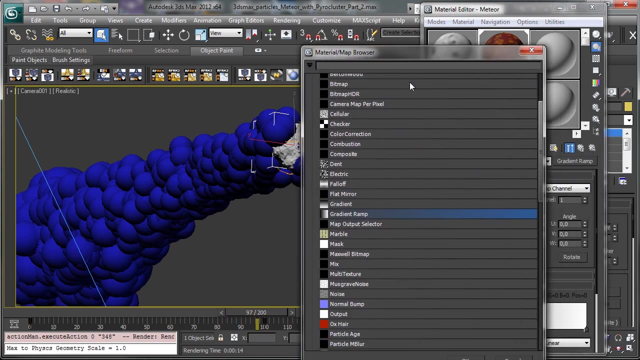 Noise And we'll have Darker red And an orange, Let's say with a fractal, Something like that, And let's see the first one scaling okay, and the second one we'll have maybe- let's say sorry, another noise. 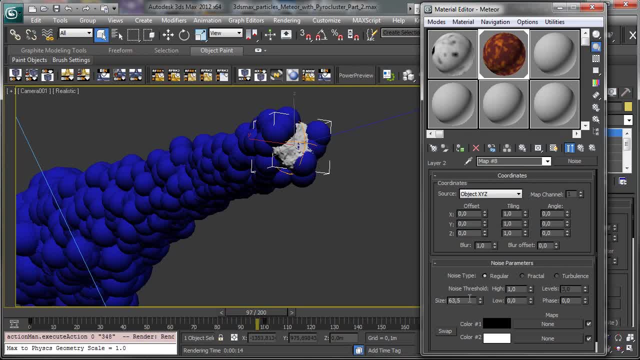 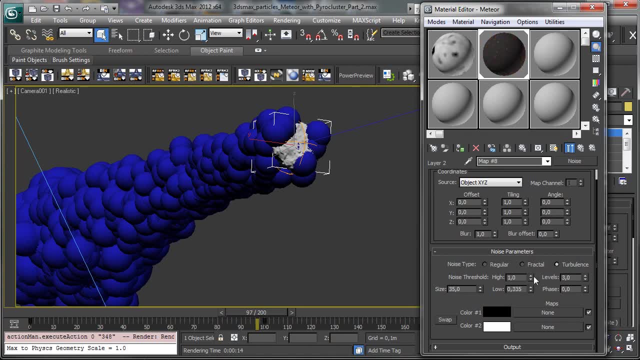 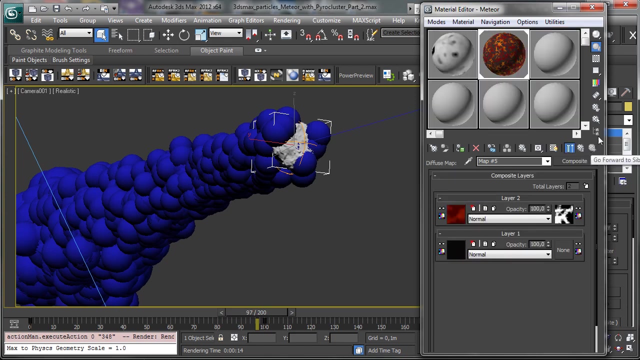 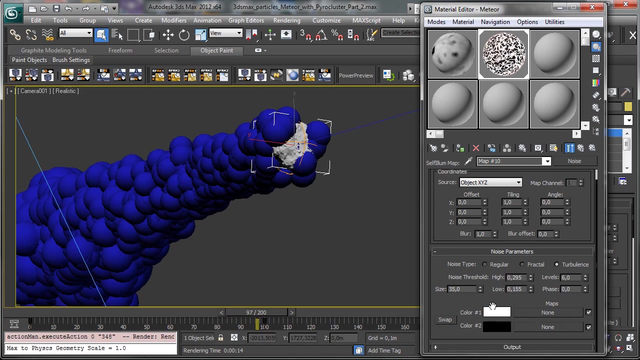 discard and we'll have maybe a 35 turbulence- and I'm just playing with the parameter. let's say 60 and their copy and let's put in the self illumination as an instance, but we need a little bit less, so let's say clear paste as a copy. 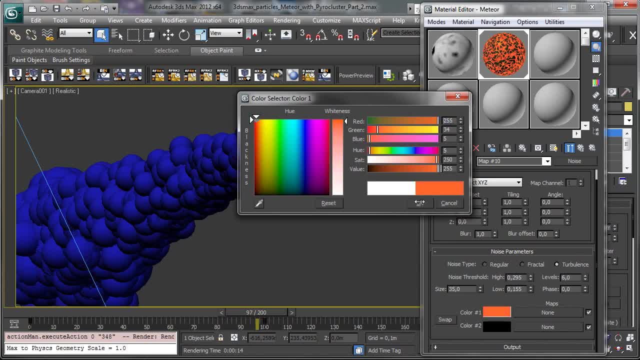 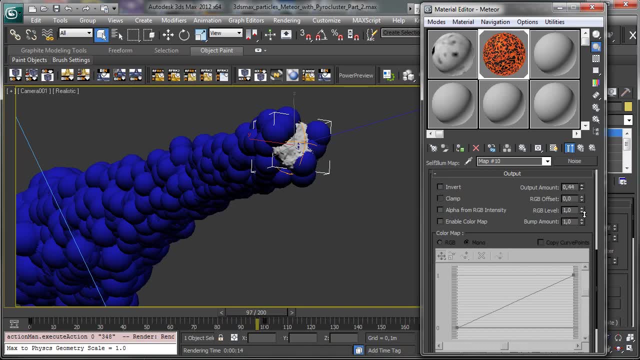 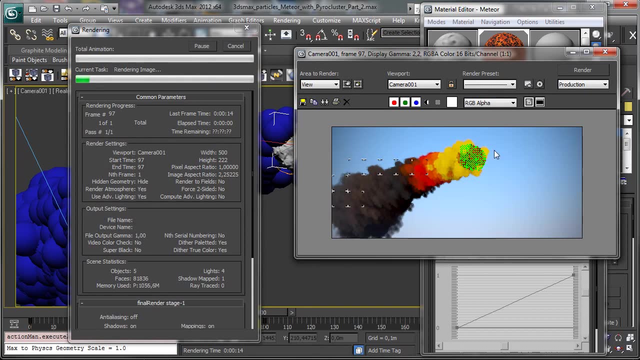 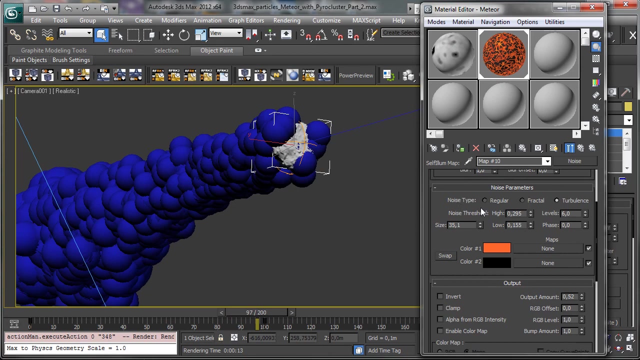 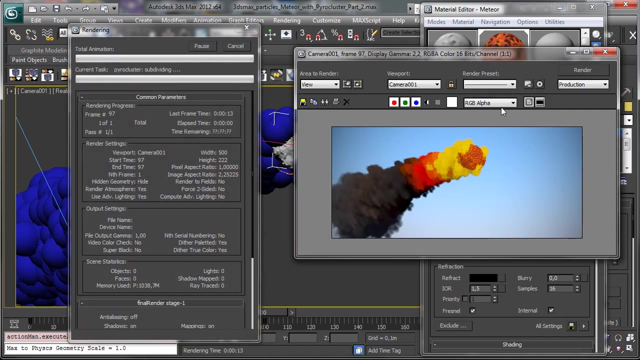 and we say something like that and black there and the output will be lower. let's see what we have inside the rendering. we should have something there or the rock, just to edit something. okay, we can change the scale. let's see, maybe 85. sorry, let's render just this area. 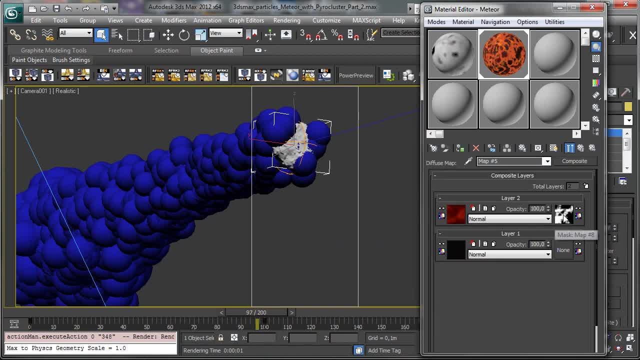 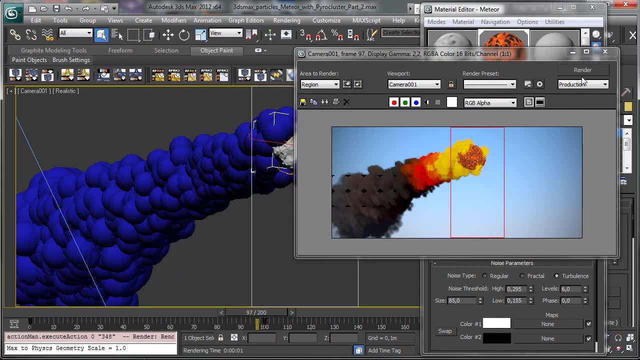 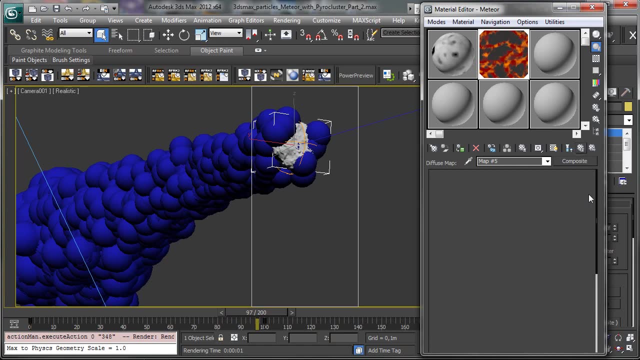 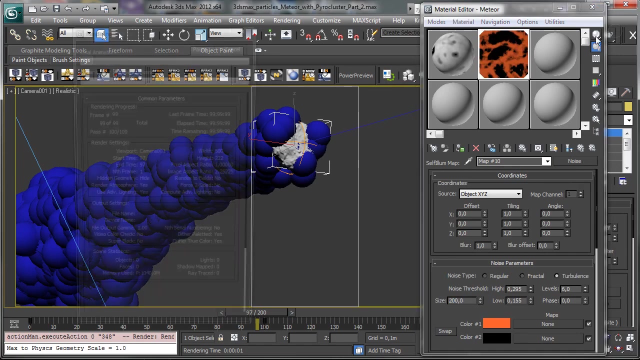 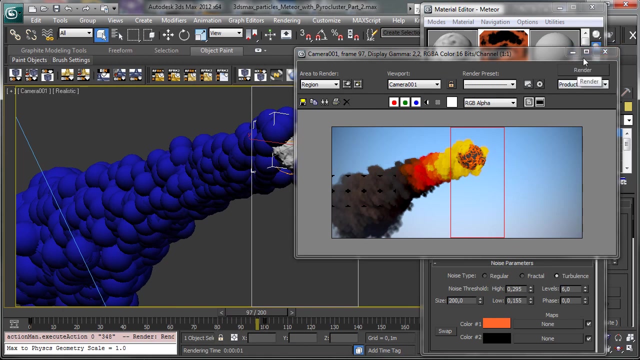 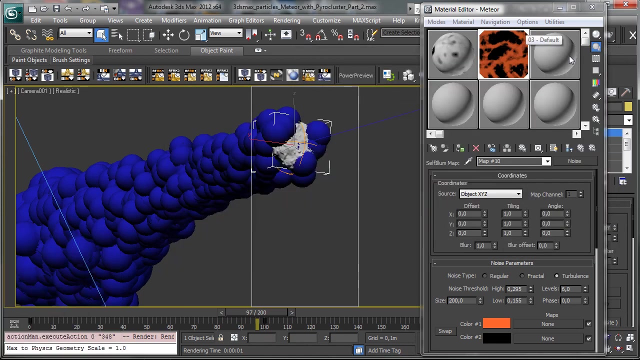 okay, let's say that also. there we have 85. we can do something bigger. so let's say 200 and 200 there too, okay, you see, we have something like that and it will be enough to have just a strange look there. okay, obviously, to have a really good quality, we should add. 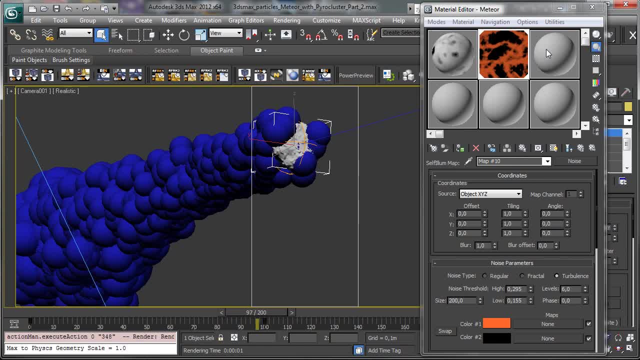 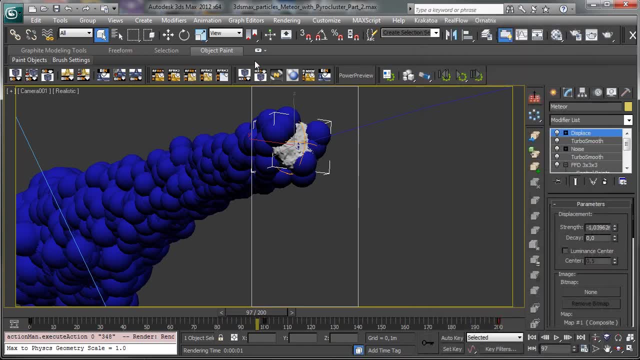 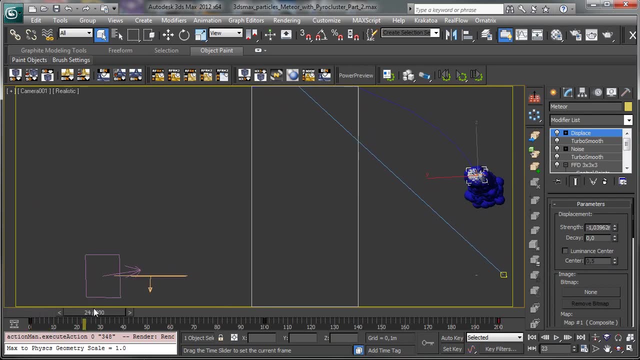 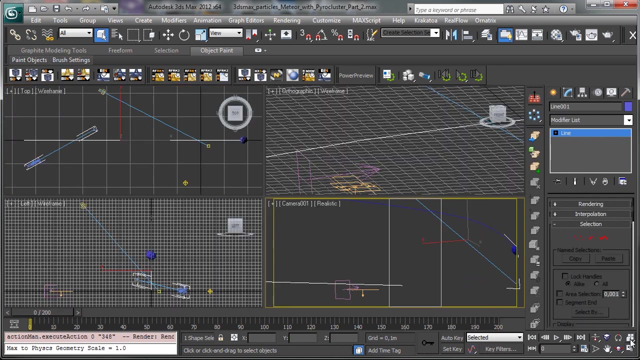 more details as the breeze, some crocodile layers and some few effects layers, but it is just to see how to play with pyrocluster to have something like that. so other thing: it will be useful to have the trail before we start there, and to have it we need to play a little bit with the line. so let's go in the front. 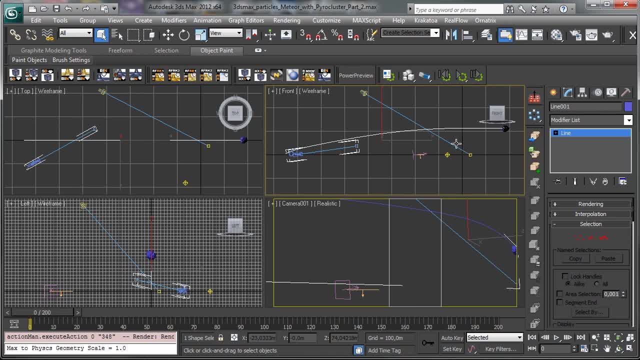 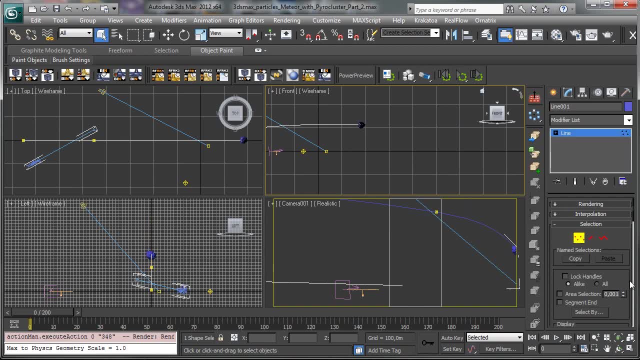 view, that's our line and we should change the line and I mean we have to refine it. so let's give the year and let's see refine and we can select this vertex and there is something like that. so you see, we have two particles: start in there and 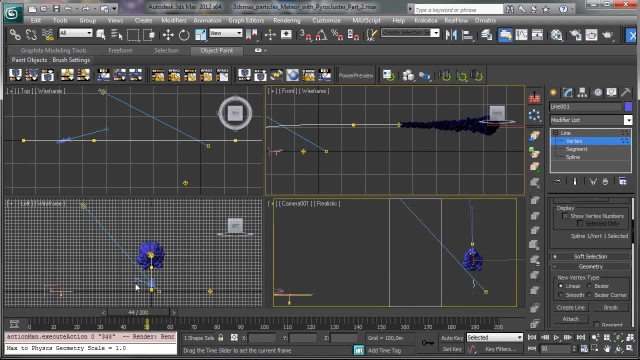 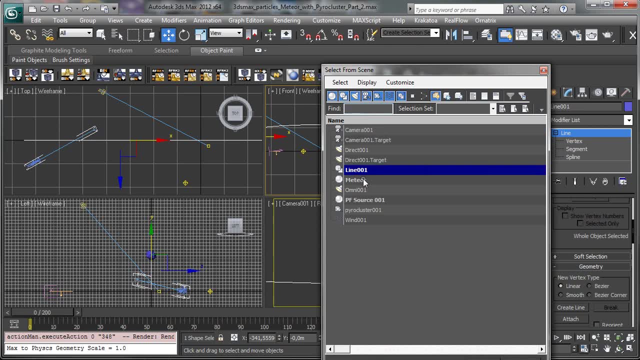 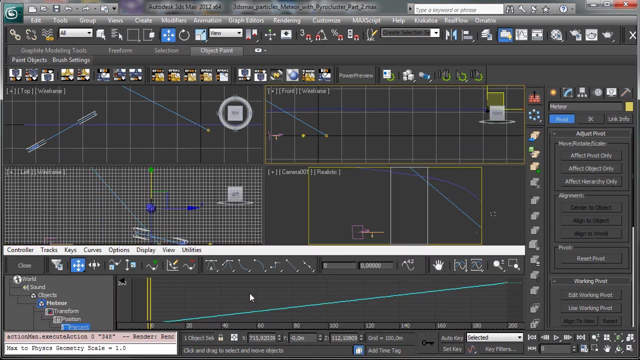 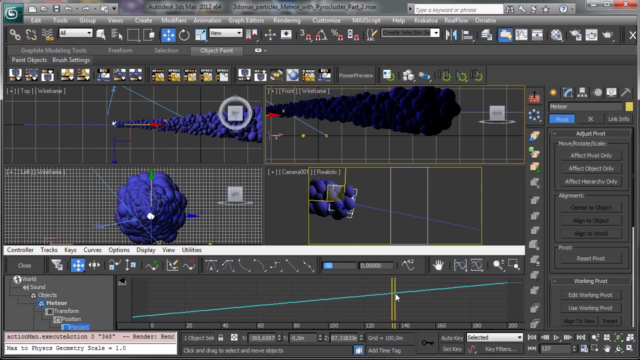 going and going inside, but the important thing is say that the asteroid will start to play with the path before you see that actually we have the zero at zero frame. let's say that this key is at minus 25, minus 50. you see, we have smoke inside the viewport before we have to. just a little. 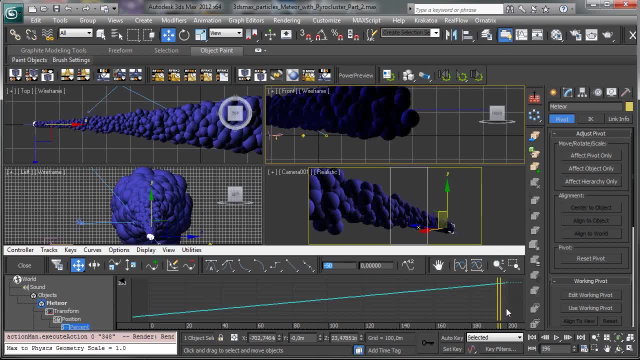 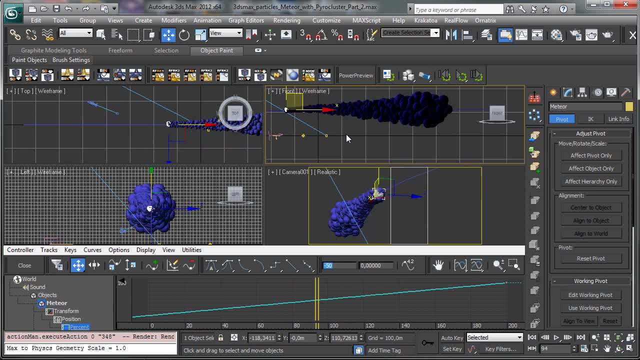 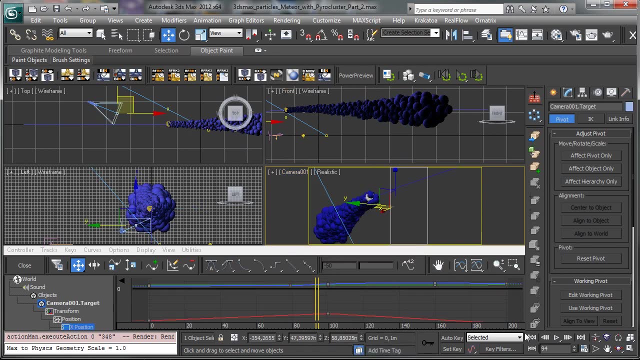 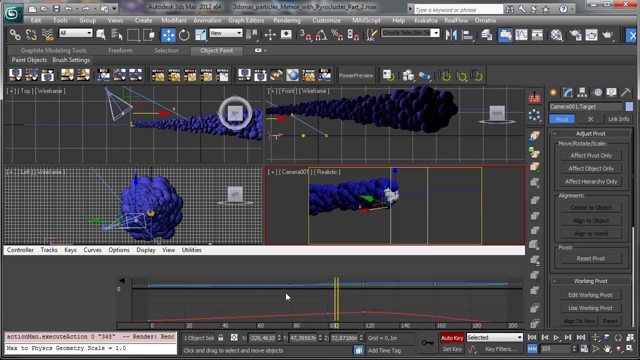 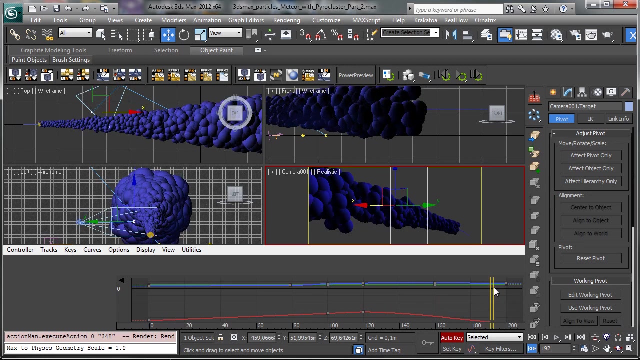 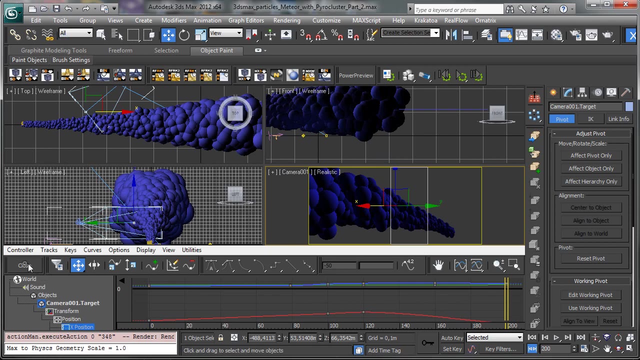 bit the camera animation. so let's go back and let's select the target. let's go key by key. there it is right and there it is not right, so let's go for the auto key- okay, this can be not bad. and let's save and close. I like to see how it looks from this. 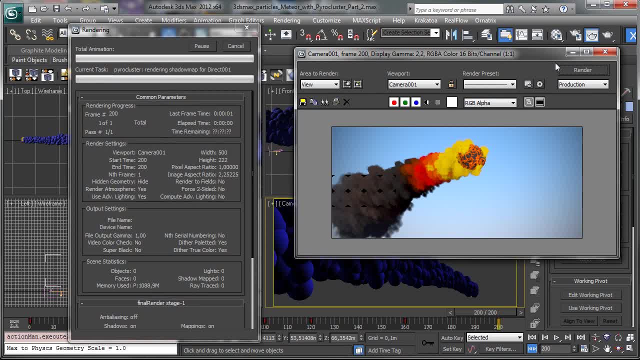 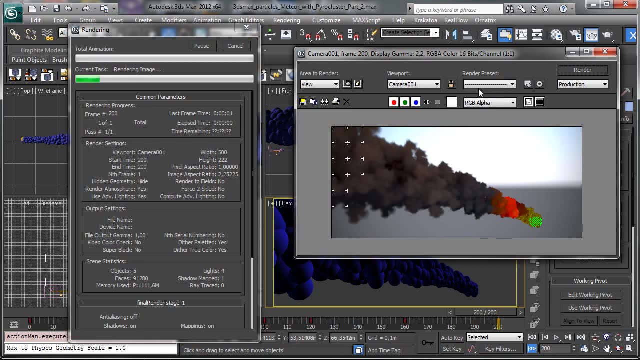 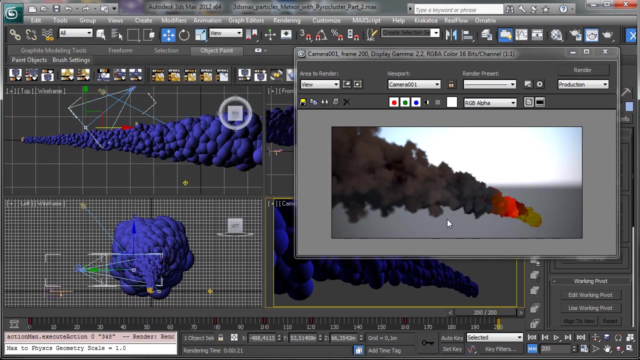 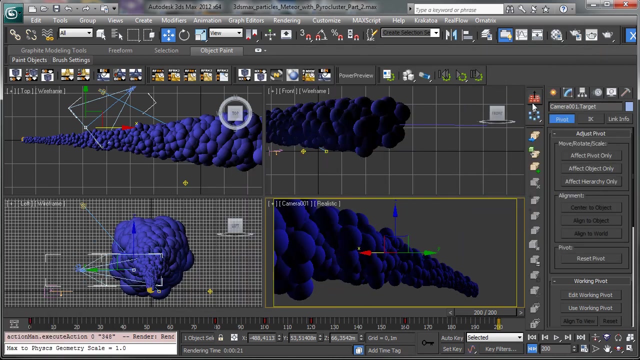 point of view: okay, okay, okay. there it is a little bit strange, but it is due to the, to the particle settings we done. we have to check another thing and that's the, the scaling there of the particles, and I think we need bigger particles at the end. 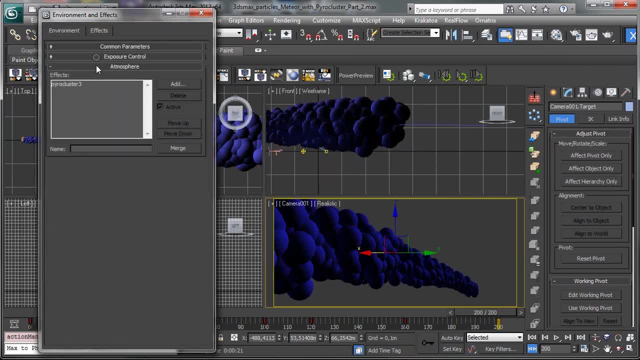 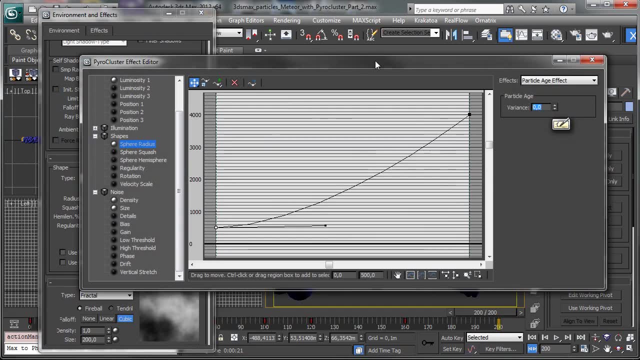 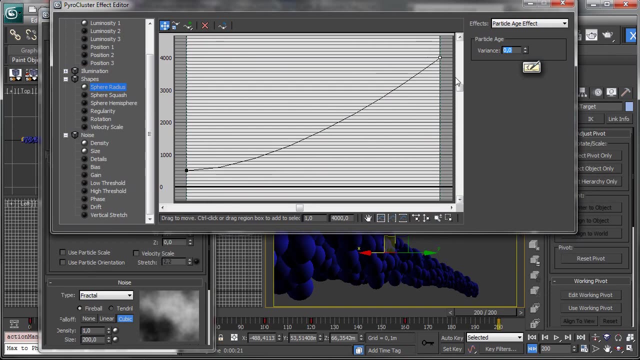 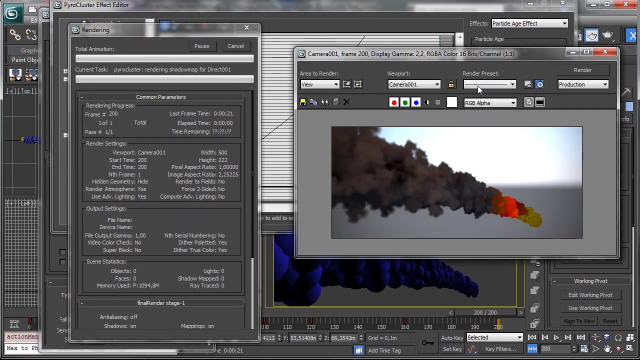 so let's go in the pyrocluster again, let's check the scaling there and let's say that at the end we have 6000. so you see there are bigger, maybe 8000. let's render again. we should have a better scale there. 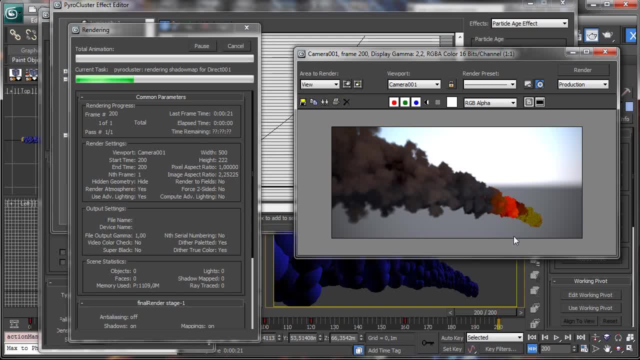 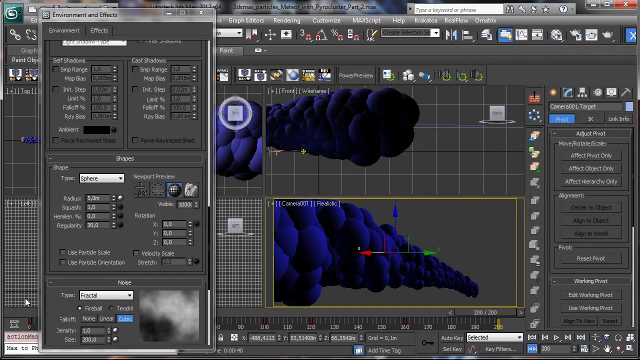 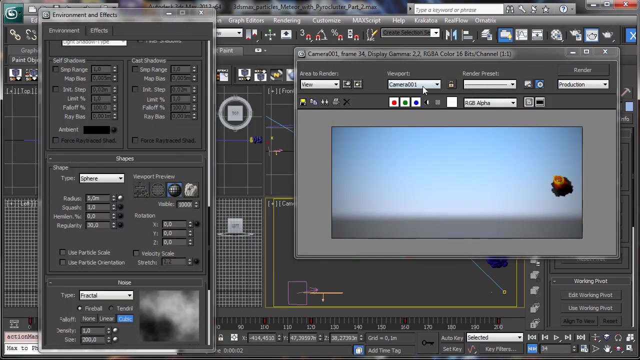 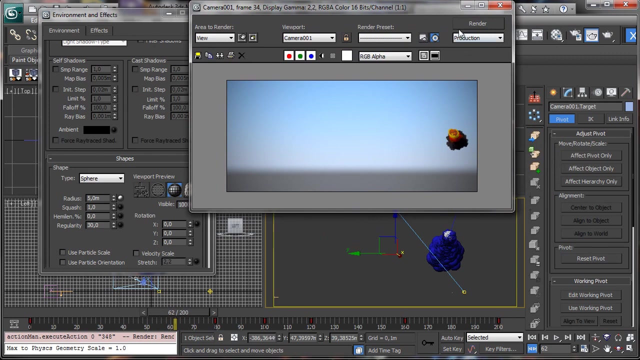 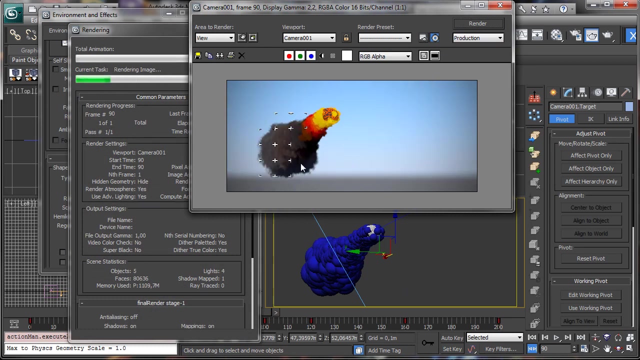 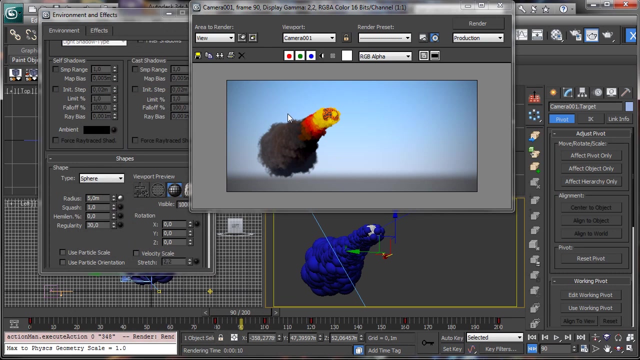 maybe we can speed up a little bit more the shadows there, but now the look there is ok and we have just to check there. so let's start again to see how it looks at different frames. I'd like also to see the density falling. obviously you can imagine that. 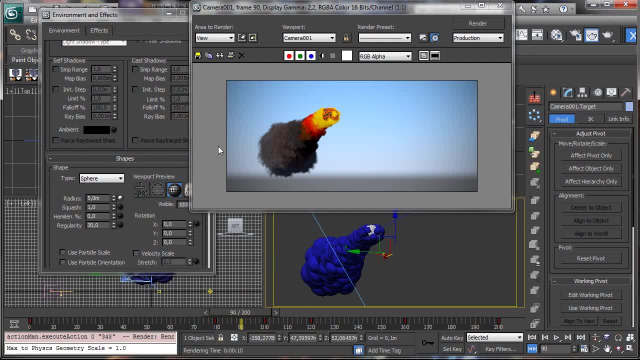 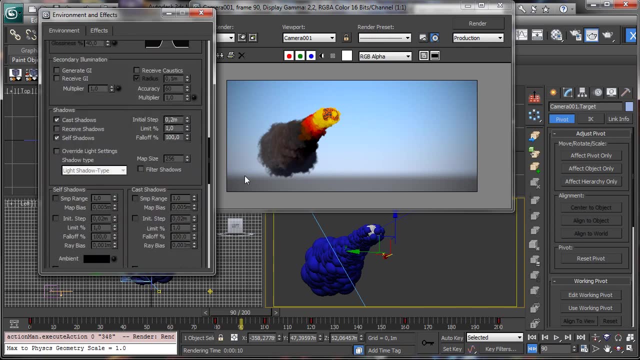 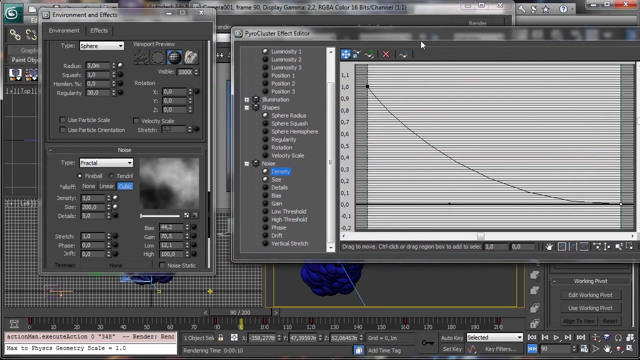 you should have a better camera position, because there I have still too much smoke at the beginning. let's go inside the density. I'd like to see something, something. so let's see how we are playing with this density there and the detail. we have still the same detail. 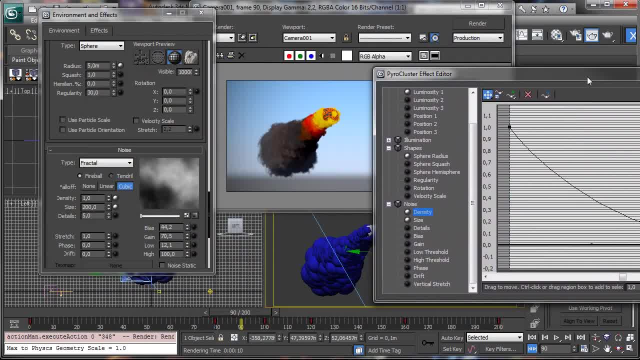 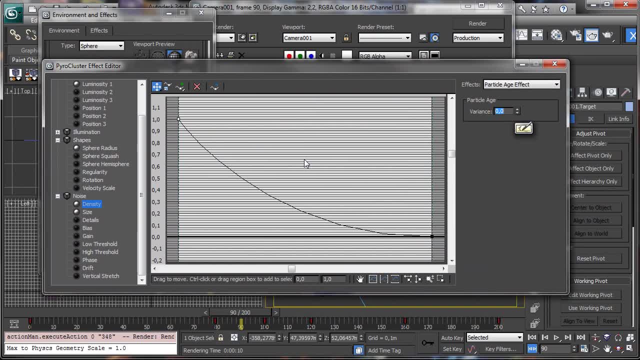 maybe we can have more detail at the end, but for the moment we see that there we have one for the density and then we have a lower density there. let's try to see what happen if we speed up this process. let's render the same. I made a copy. 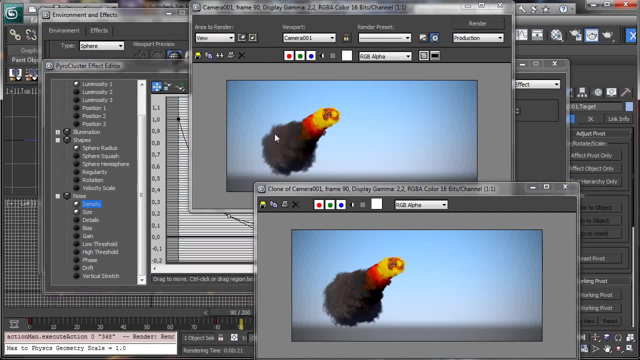 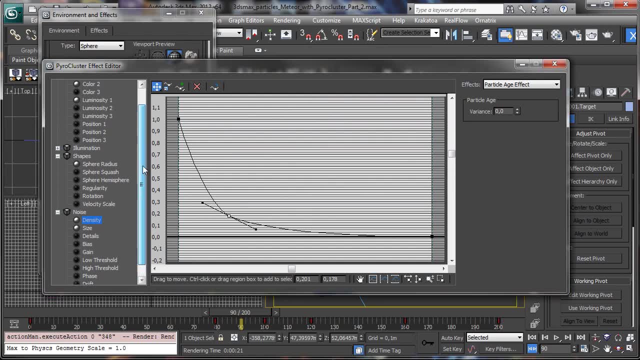 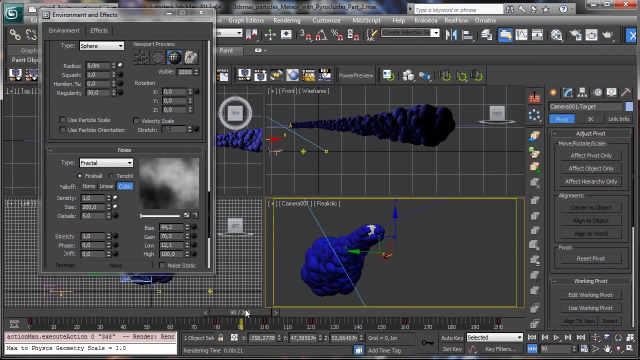 ok, you see that we have a little bit less density there. I'd like to see if there is something more I can do. let's see what happen from this point of view. let's see what happen from this point of view. ok, let's see what happen. 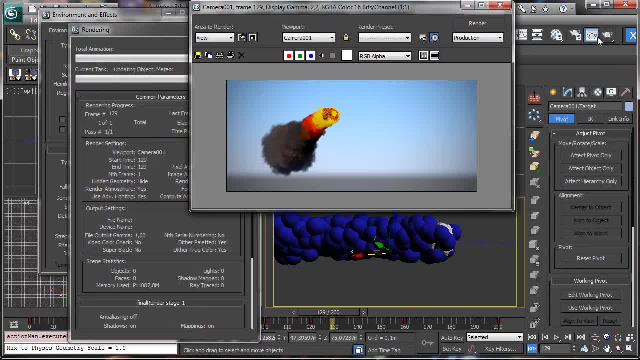 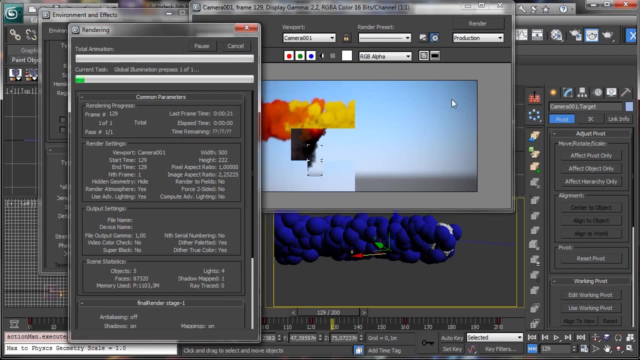 from this point of view: ok, let's see what happen from this point of view. ok, let's see what happen from this point of view. we have to speed up the shadows, maybe just a little bit, but we have to do it. ok, you see, that's what we have. 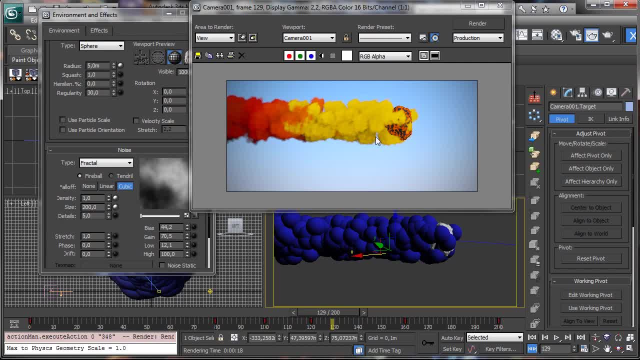 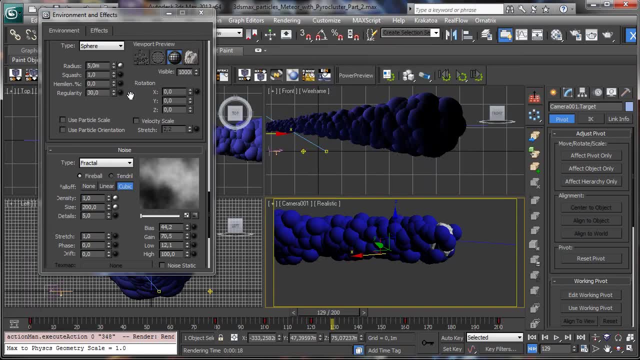 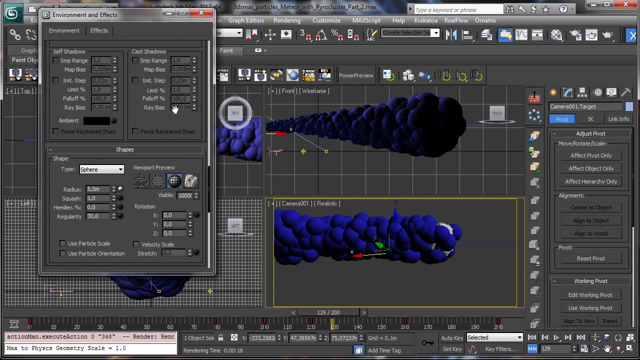 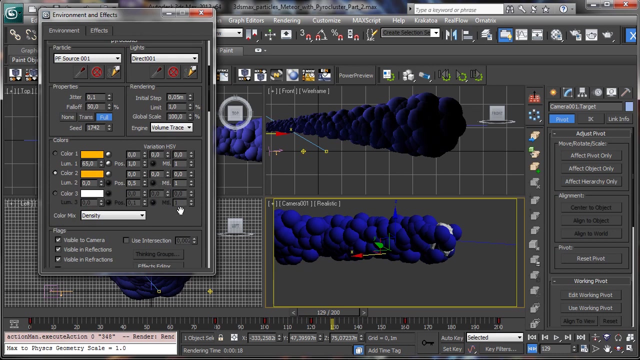 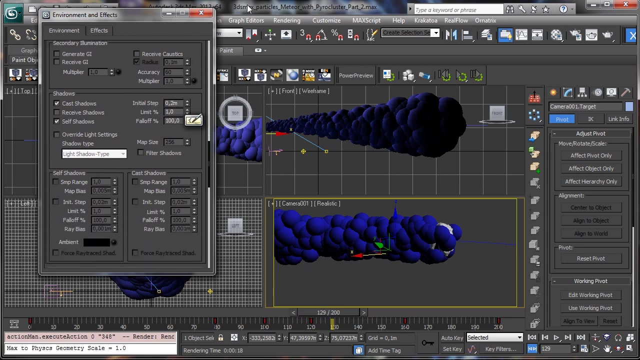 in this part and we have still not so good amount of particles. so actually I think also that we are using just some particles and not all the particles. let's go at the beginning to check and before I like to go there and let's say that there we have. 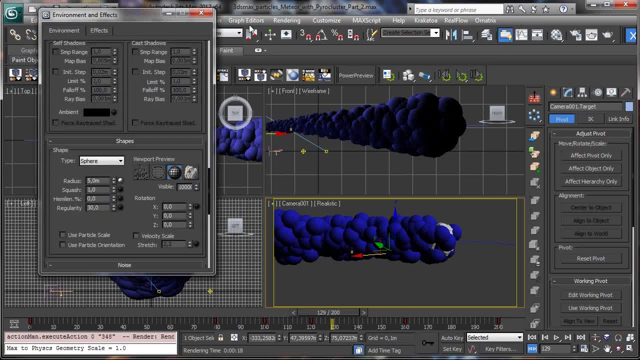 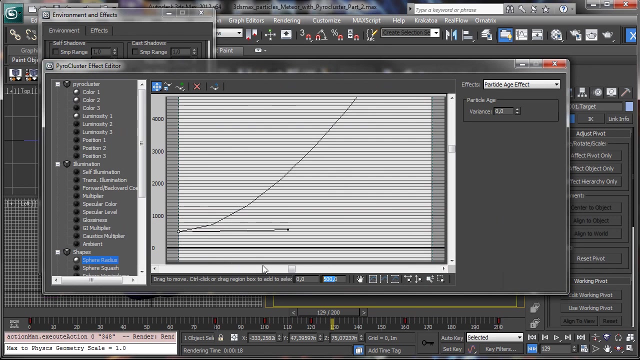 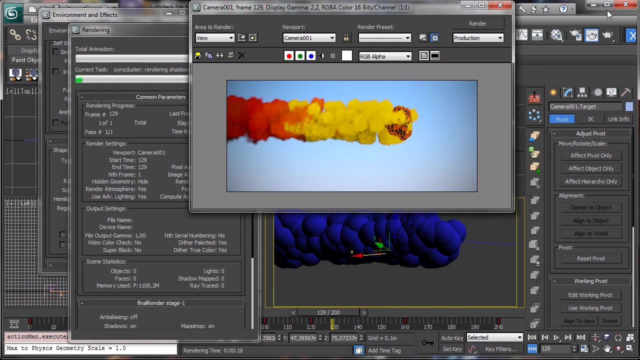 0,3, so it will be faster, and the: I think we have to play a little bit there with the scaling so we can have the radius there we have 500, let's try with 7500. maybe it will be not more visible, but sometimes between 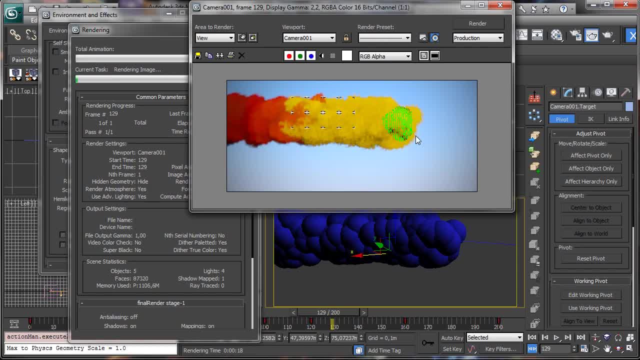 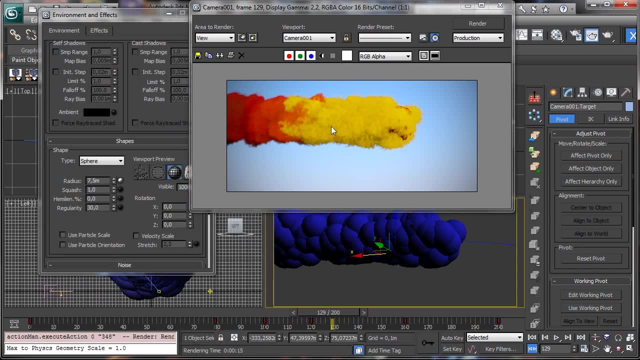 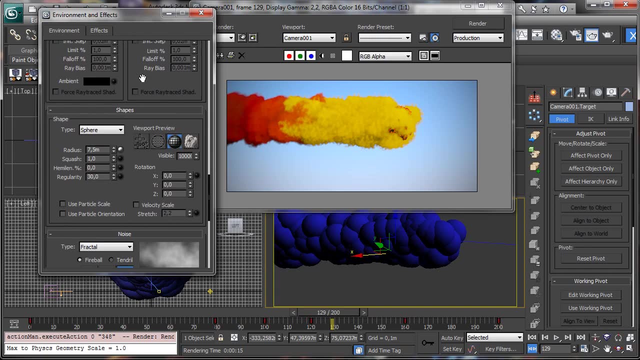 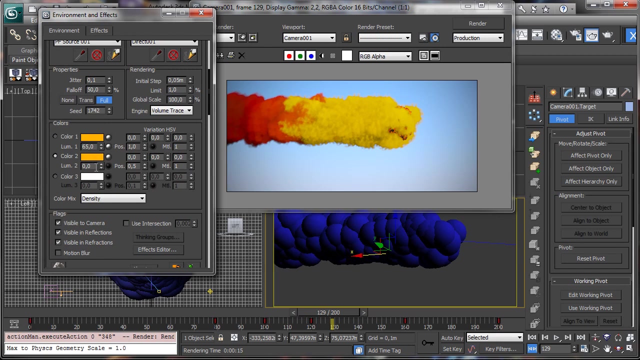 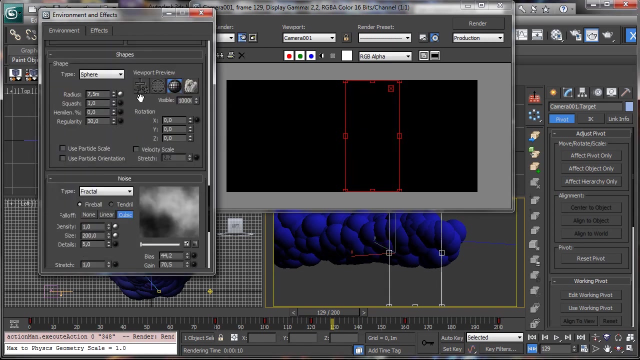 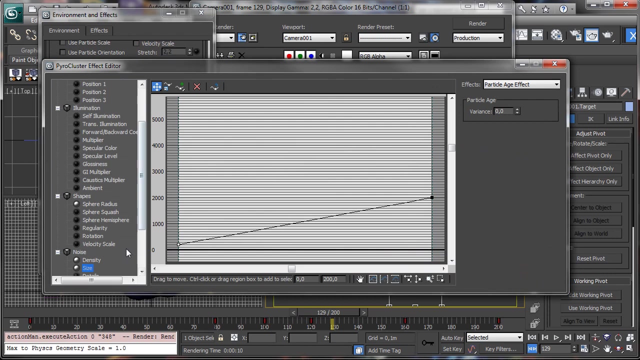 the volumes, we can see the rock and we are seeing better also the scaling there for the, the noise. ok, I think we have to play more. I like to scale a little bit the detail at the beginning and we are there. so let's reopen. we have 2000. 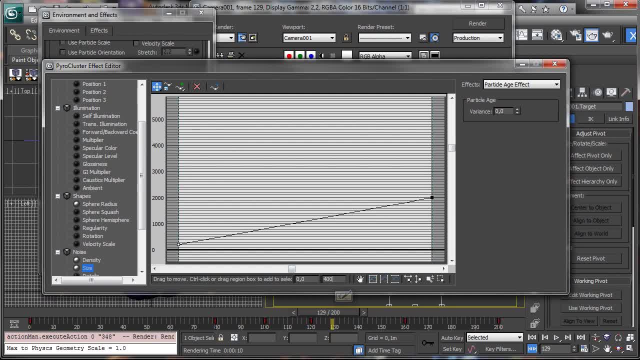 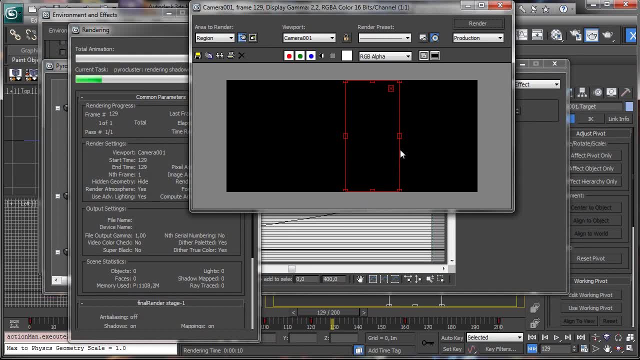 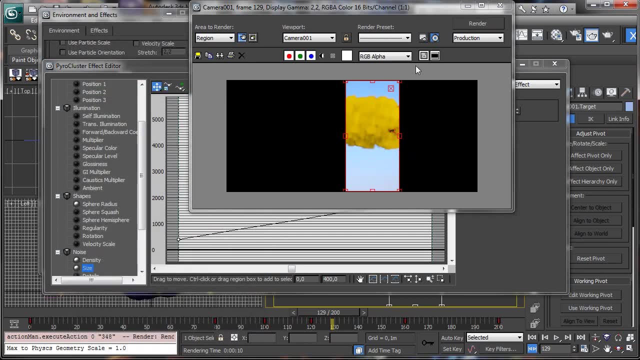 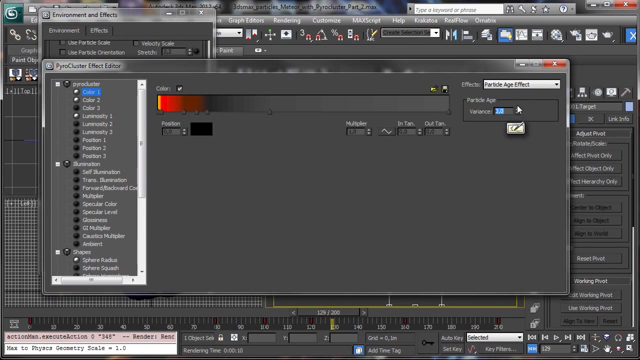 there and let's say 400, because we had not so much detail before, but now we have too much detail. ok, you see, it's a little bit better. I like to see again the color. let's see 12 a little bit of, let's say maybe. 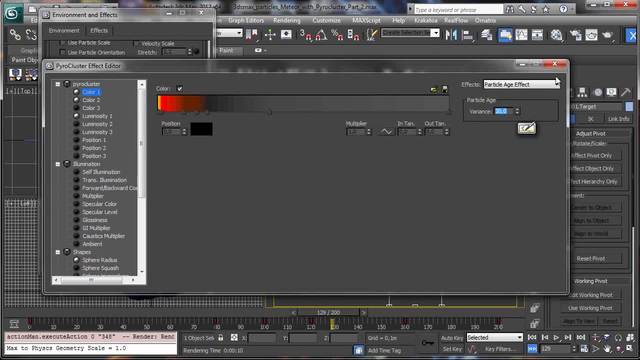 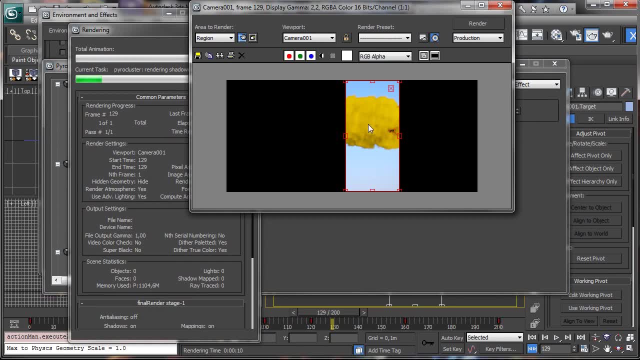 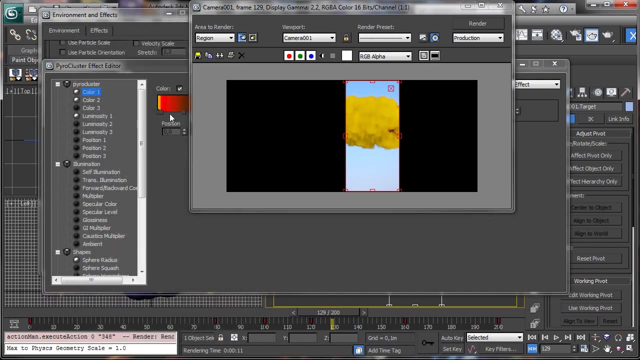 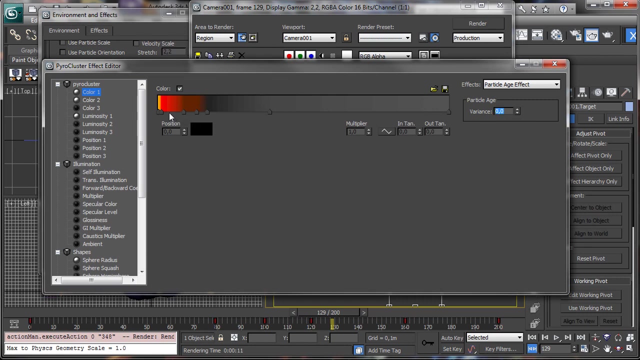 an eye value, just to see how it looks. it is not so useful actually. I prefer to play a little bit with the coloring, and there we have too much. let's give 1, sorry. 2. ok, so it's really near to the second one. ok, let's check the second one there. 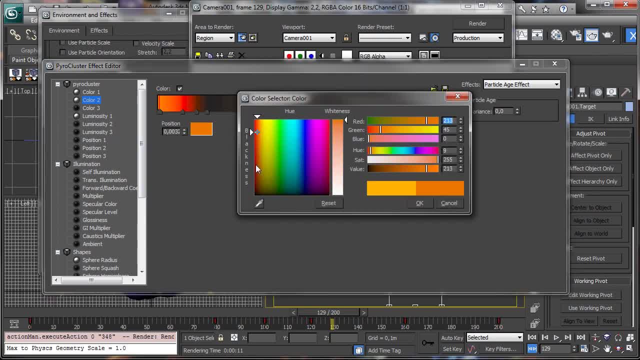 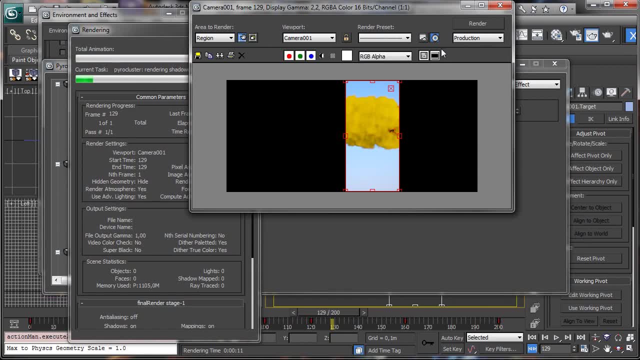 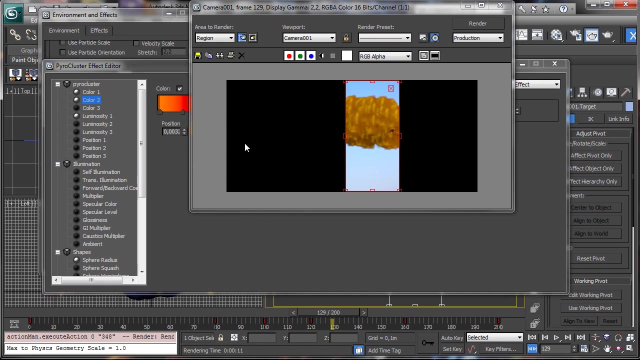 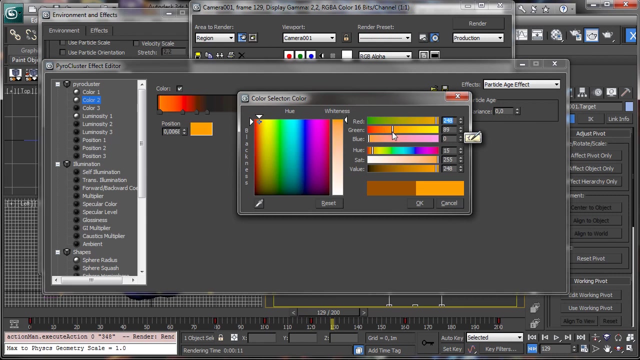 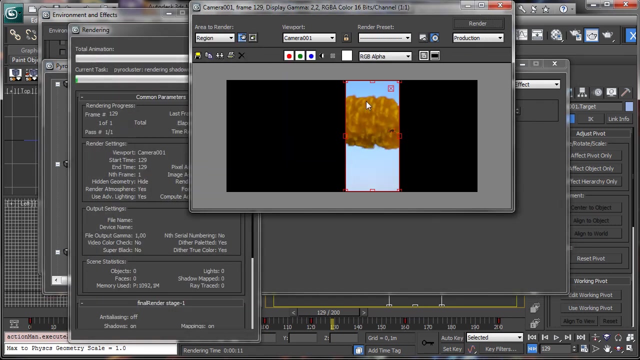 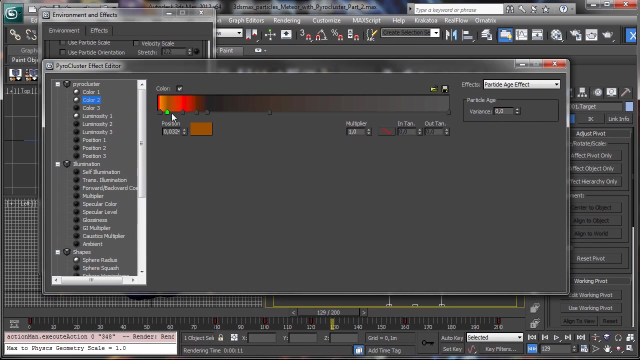 and let's go for a more darker red. ok, you see that now we have the right strange coloring there and this one is not so so good. so let's go for an orange to find the best coloring there. we are still this color. let's see in this way. 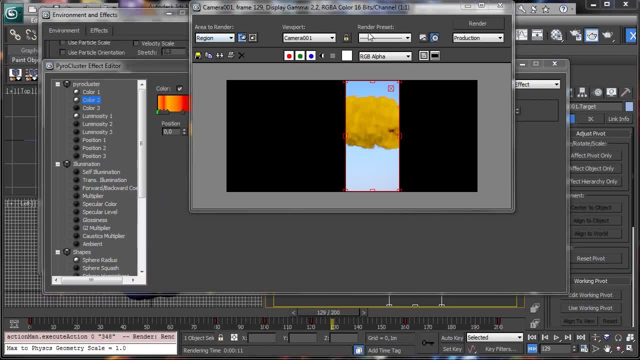 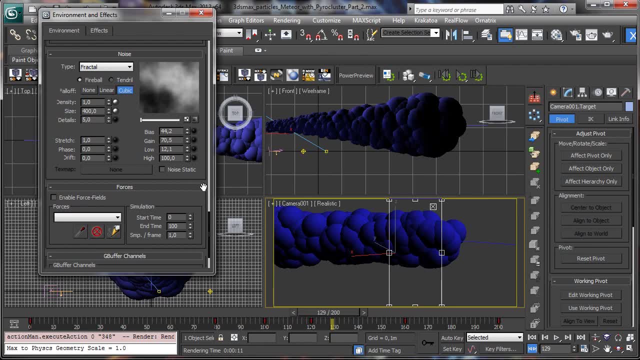 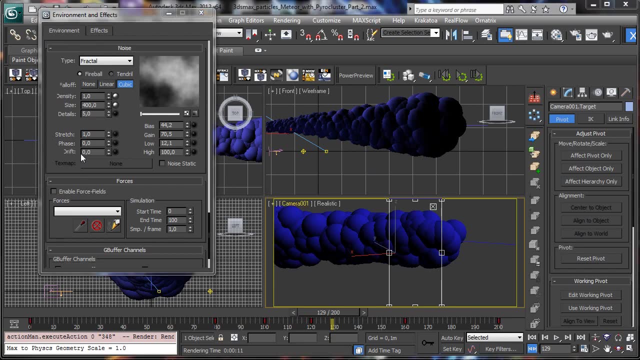 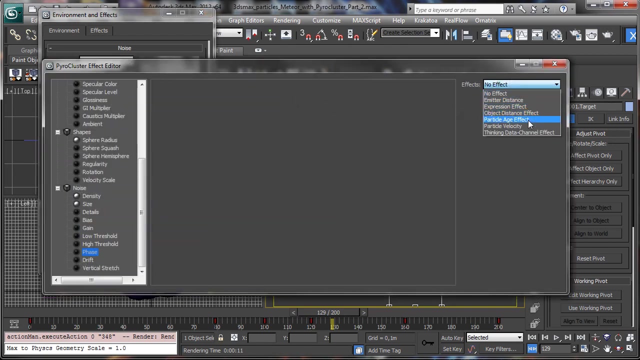 ok, we are back at the yellow we had before and I like to see something there. you see that we have actually all the same orientation for the fractal. let's use a face, because you see that actually we have no animation and we have the face linked to the. 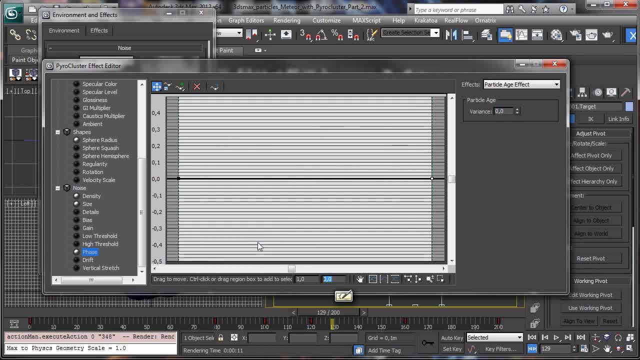 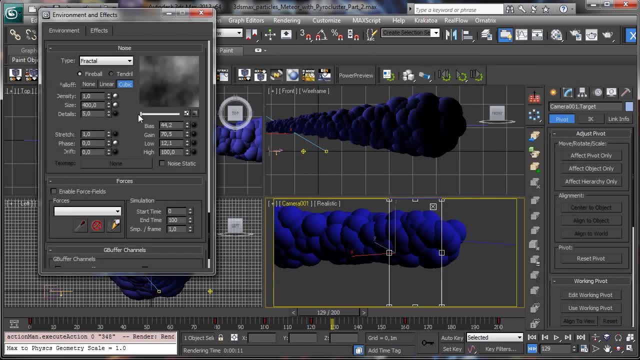 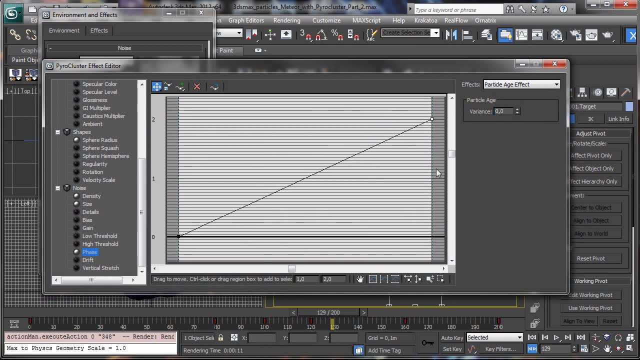 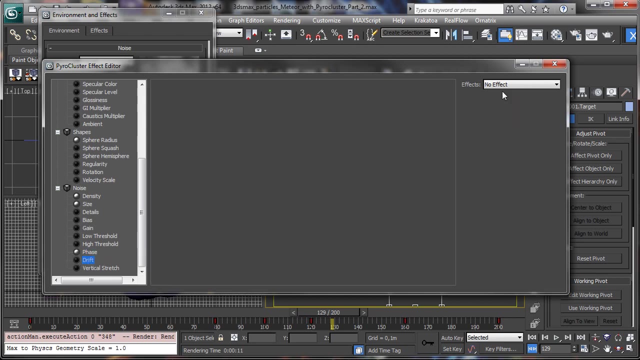 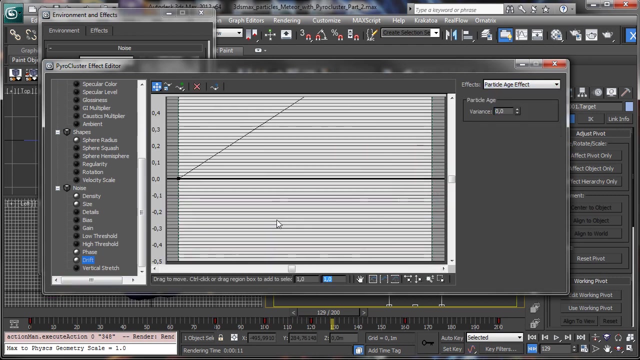 particle edge, and let's start trying with 2. so you see, maybe it's too much. we have to make some test. this one, let's try with 1, or we can play also with a drift and a drift. let's have a low value there too. 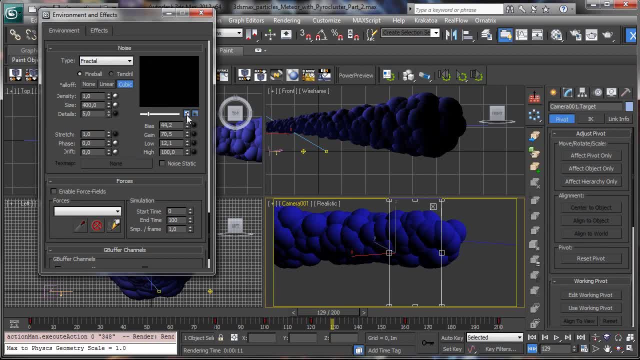 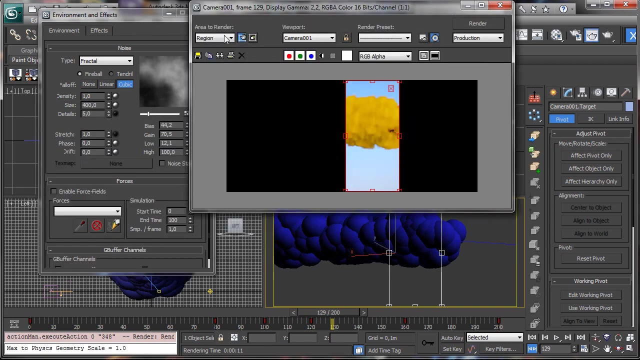 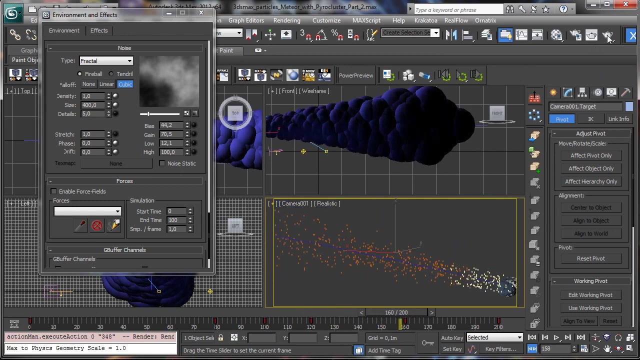 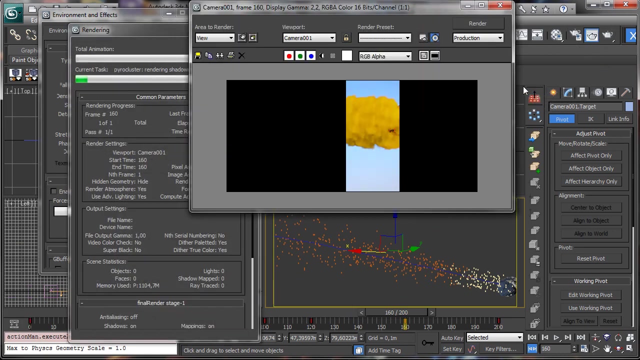 ok, let's go in the drift and let's try to have a really high value. it seems not so much, so I think it's enough. let's go in the rendering view and let's continue to check how it looks. we can still speed up a little bit. 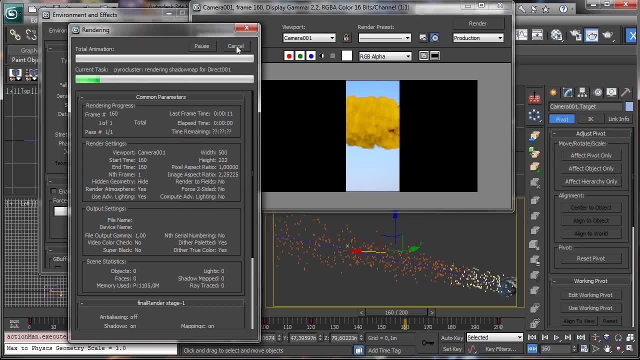 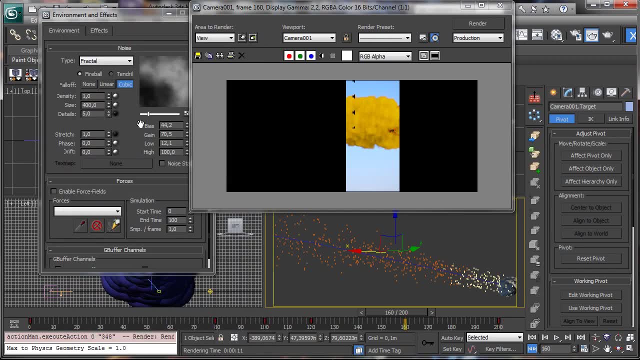 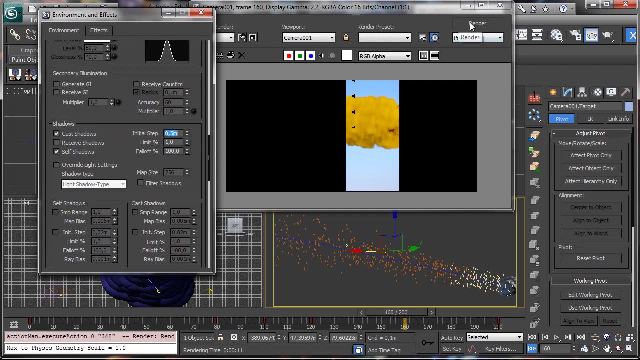 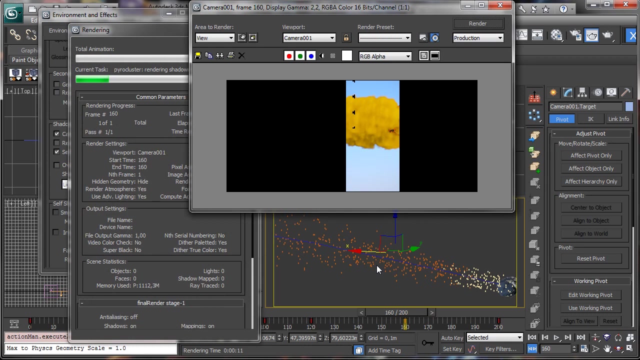 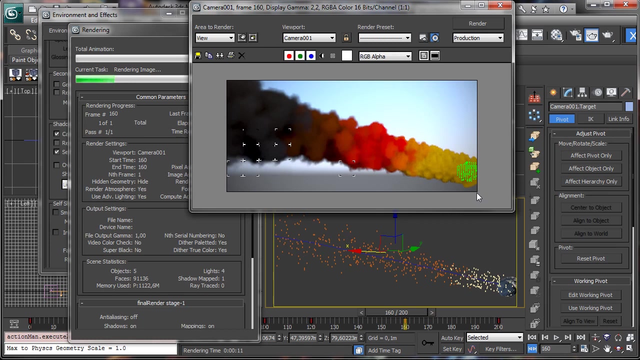 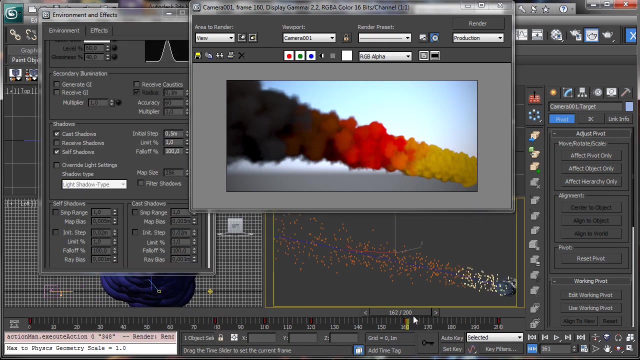 the shadows because it is too much slow. so let's go again inside the rendering and let's see to have 0.5. maybe the quality will be not so high, but the speed will be really, really better. ok, that's what we see there. I'd like to see. 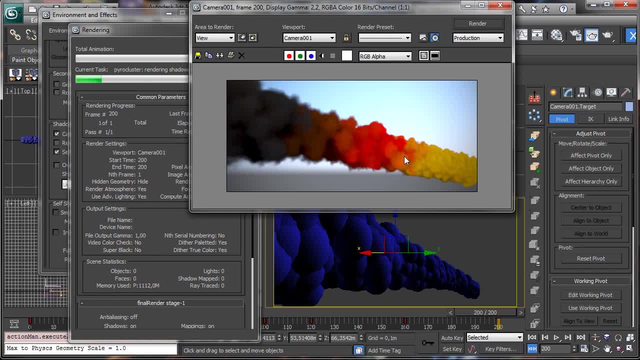 at the end if we have too much black slow smoke. so I can change a little bit there we have a good smoke there. there we have a little bit of low quality due to the parameters we are using, but I think we can use it because we left there the glow. 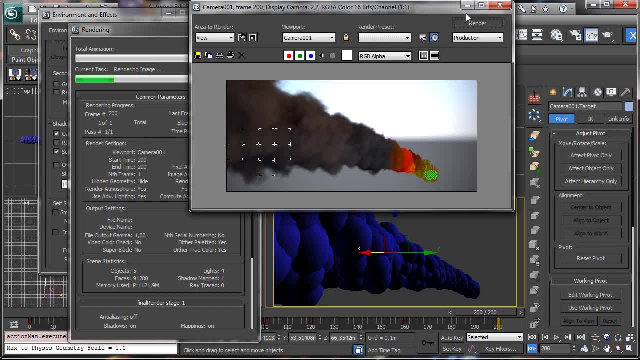 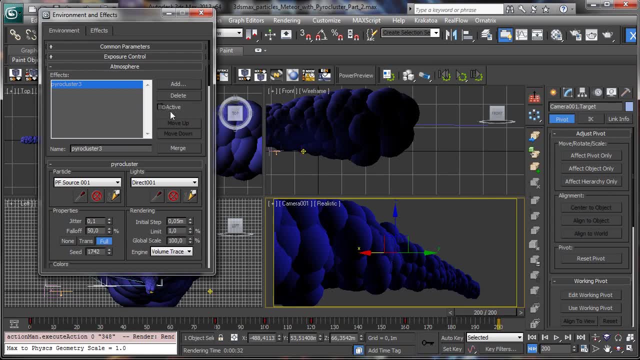 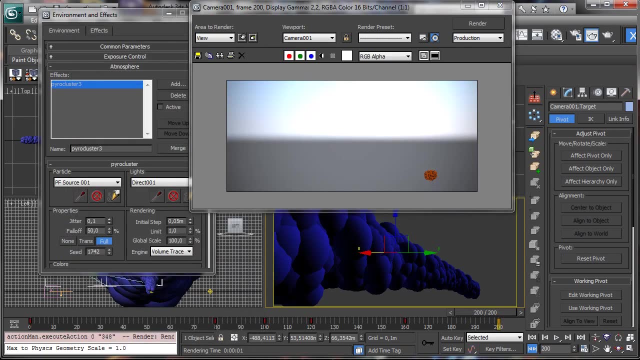 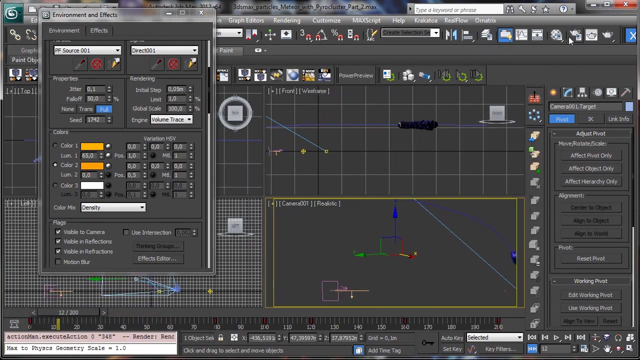 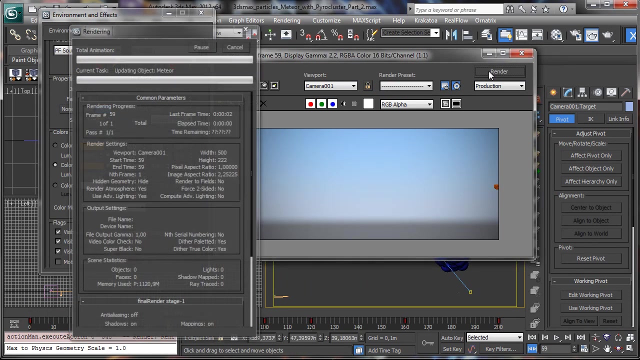 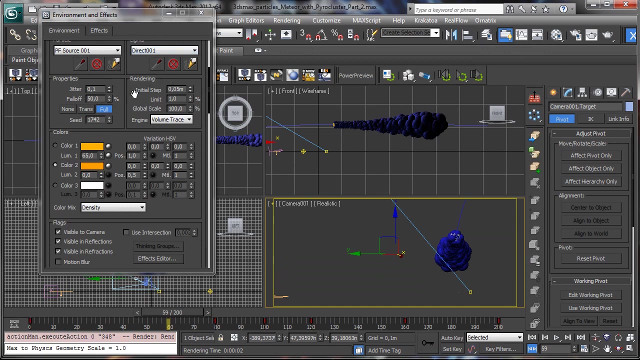 and other things, so I think this will be not a big problem. ok, let's stop and save. let's deactivate para cluster for a moment and let's see the sky. it was just to see how it looks without the dust smoke for the asteroid, ok, so I think. 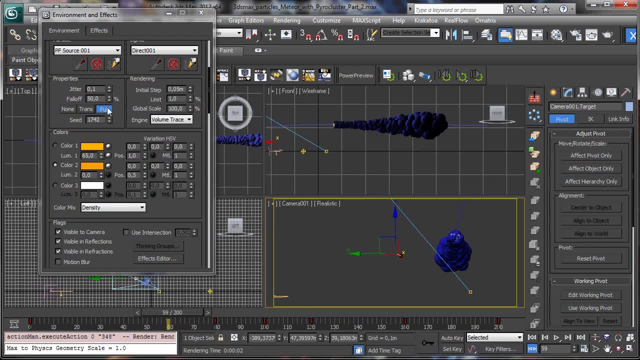 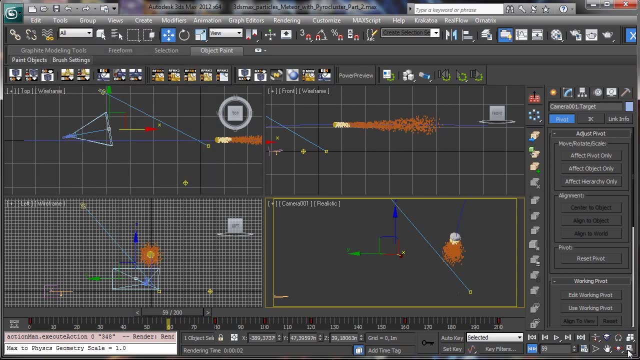 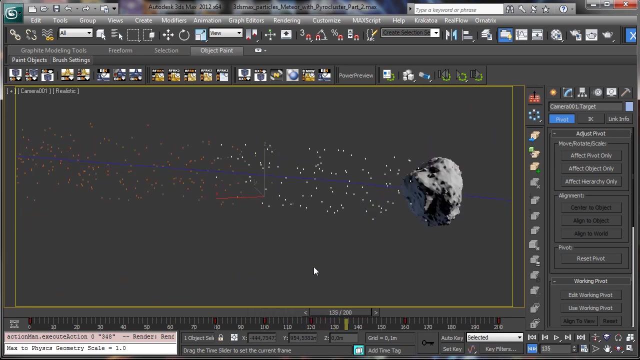 that we have a lot of good information there to have our first render, so I'd like just to see if the animation is right or not, so let's go there at full screen. I don't like so much there at the beginning, so I'd like to play a little. 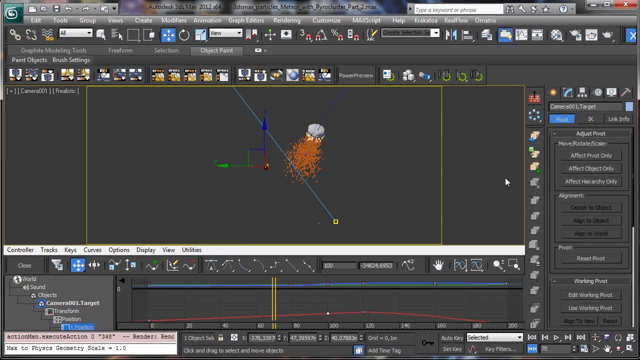 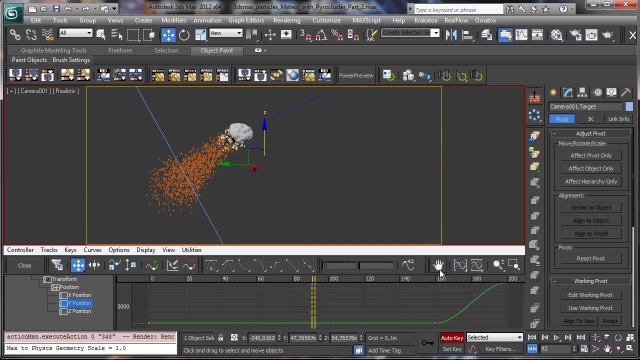 bit again with the animation. let's say to remove this one. so auto key. let's say that we are checking higher and this one will be linear. let's remove this key for the moment. and also there we have to play a little bit. let's see that we have. 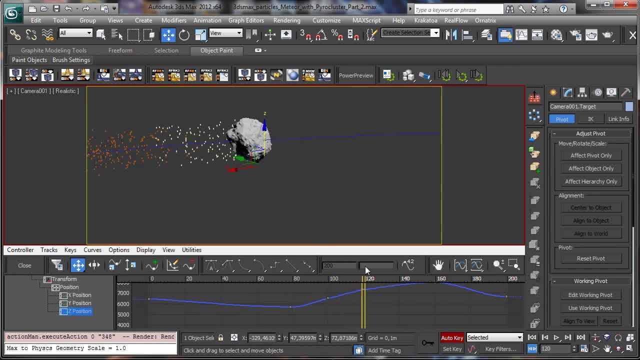 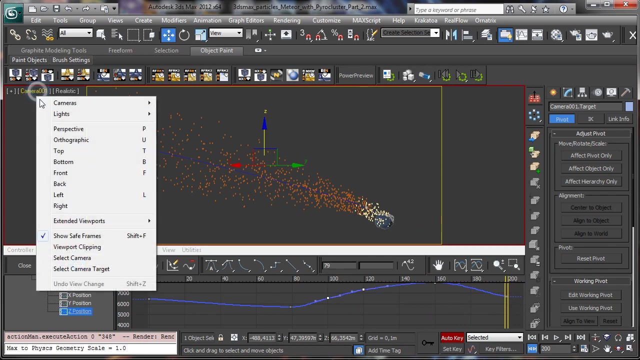 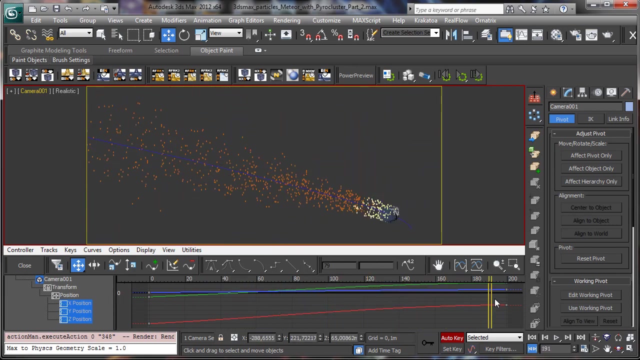 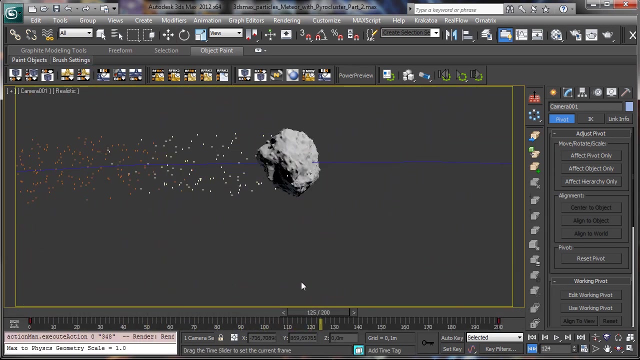 this one in the middle. ok, now it's more linear. ok, it seems a little bit better. let's select the camera and everything there seems fine. ok, close and save. now I'd like to see how it looks, so let's. 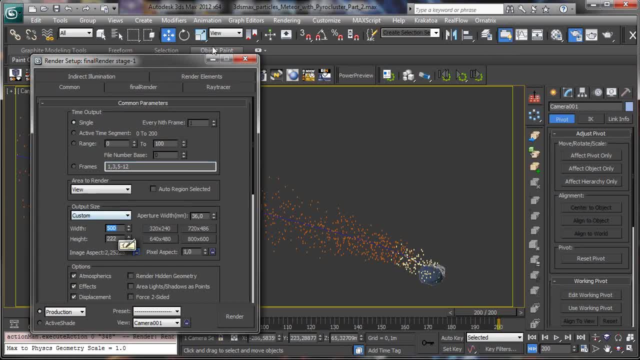 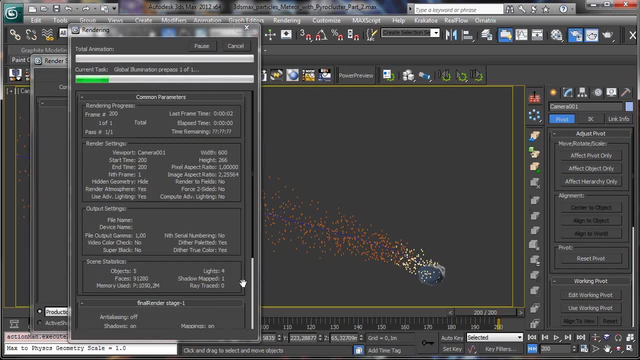 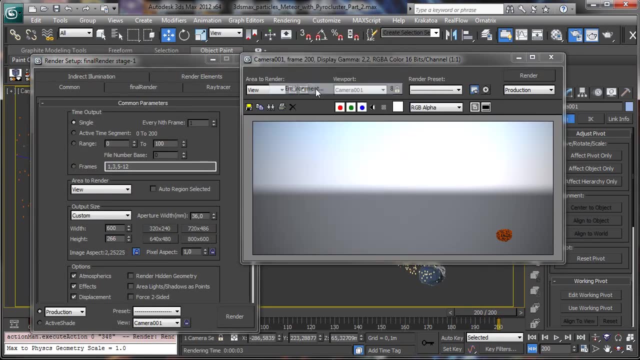 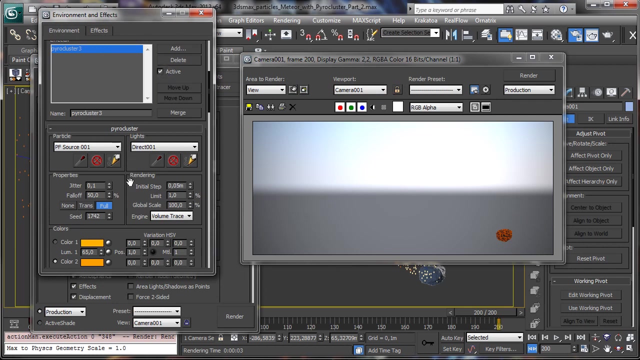 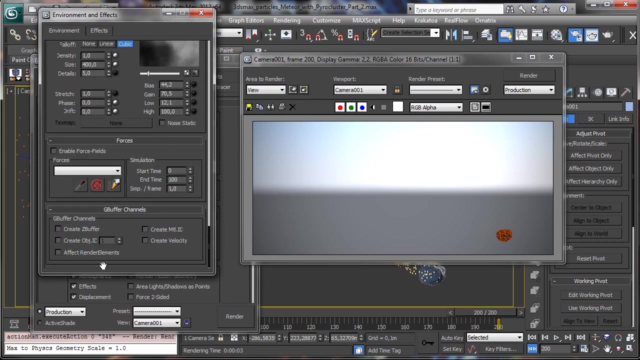 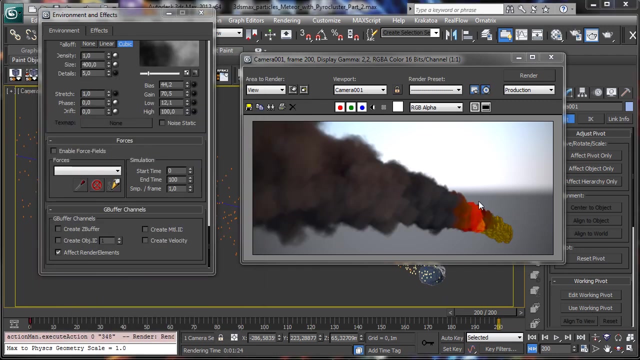 pick, for example, this frame and we make a test rendering. let's play with 600 to have a faster render export, maybe just there and I'd like to see. I think we can. 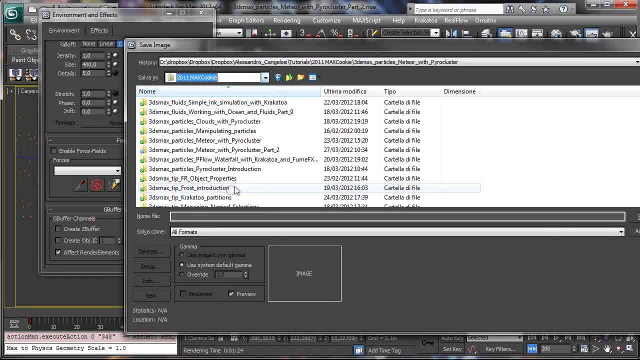 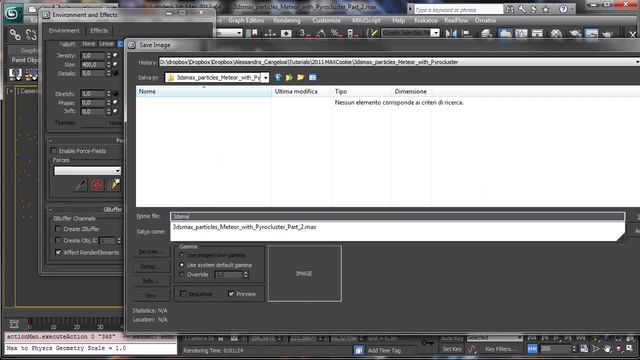 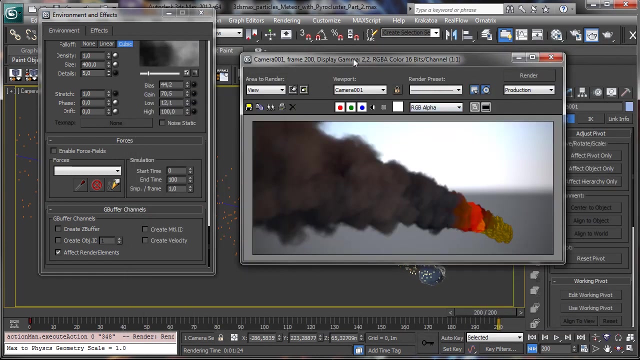 use this one without the need to render something later about the other render path. so let's call it 3ds max particles- pyroclusterpart2testtif, and we save it to 16 bits and with the alpha channel and pack bits. ok, now we need combustion. 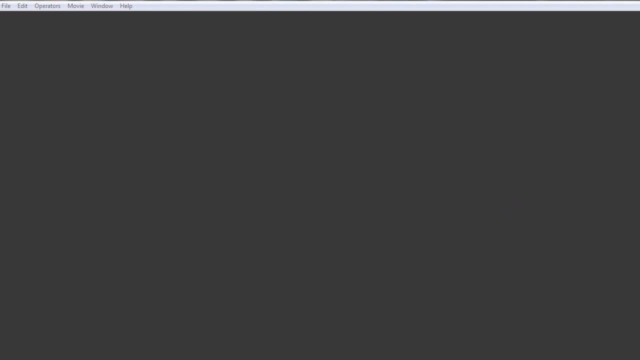 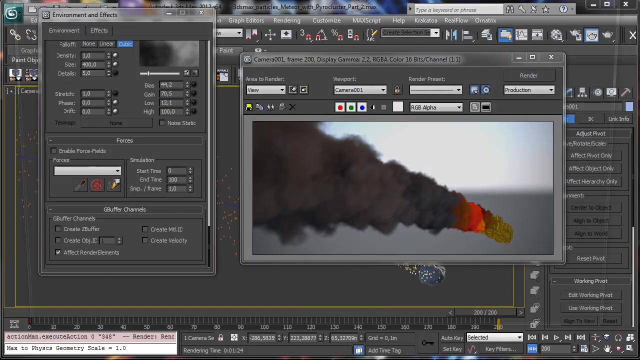 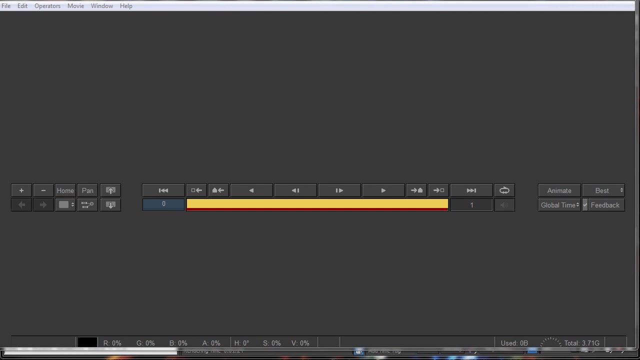 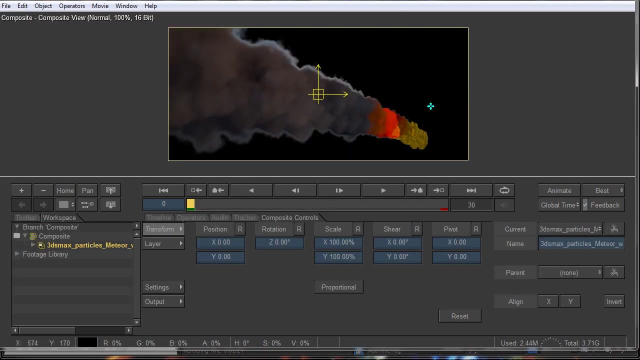 I have to scale the user interface there so we'll have the right resolution and now I can relaunch it. let's open the frame I'm doing in the other window because there is no space. so I'm going in the right folder and I'm creating a 2D composite. 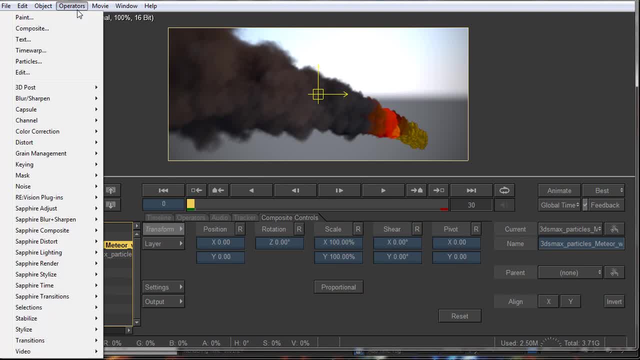 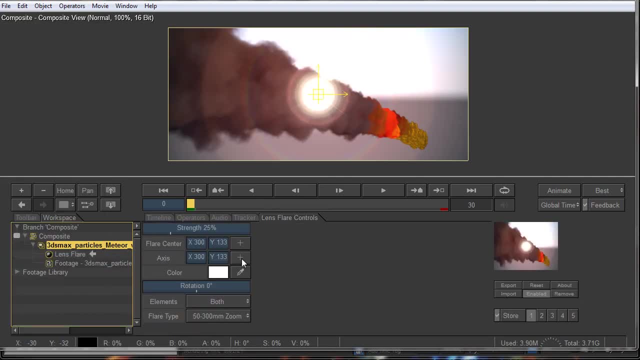 let's use all the channels we have. ok, what we can do there. first of all, let's save a flare and we'll use it there to illuminate the scene. we can try to change the color to have something different. obviously, you have to manually animate this one. 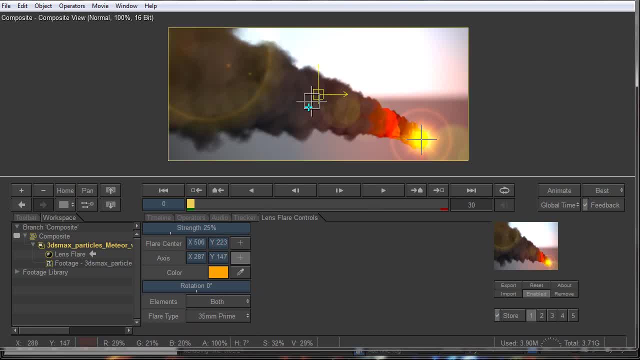 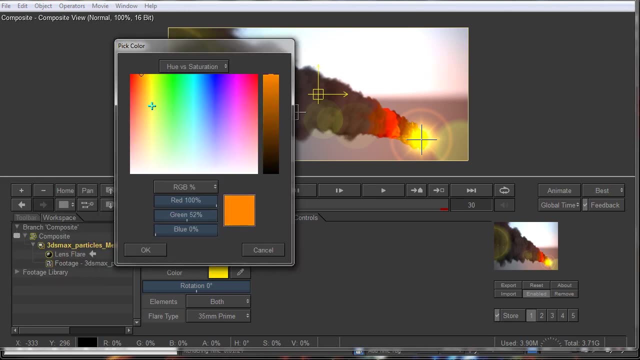 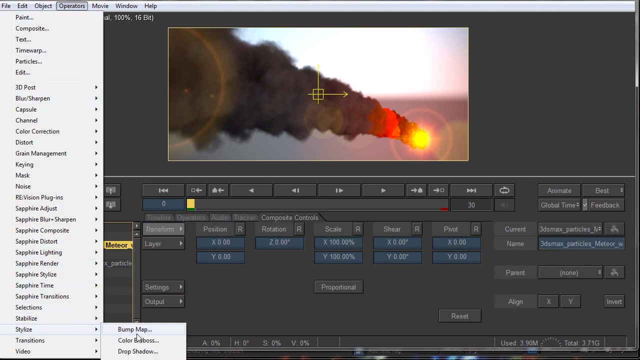 but we can use also the tracking and there we can have the secondary in this way. actually I'll play just with a- sorry, I'm changing the color- with a basic setup and then you can play with all the other stuffs in style. lights, we can use also the glow. 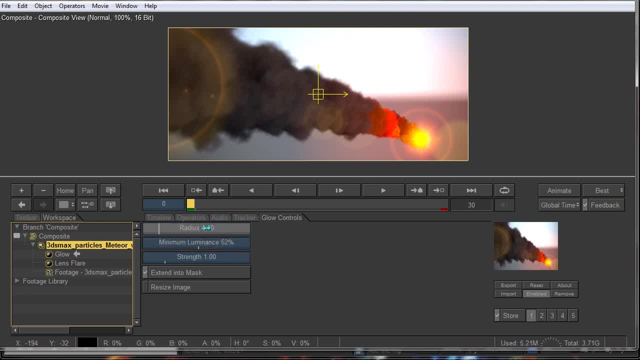 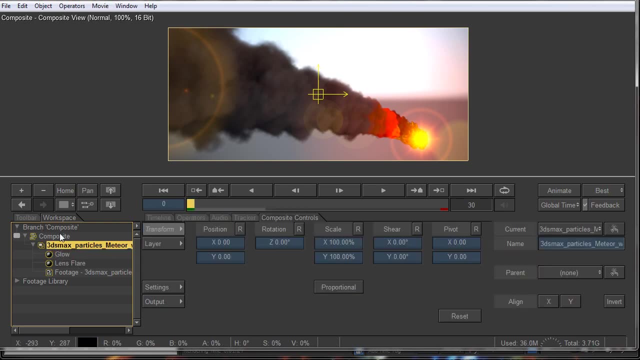 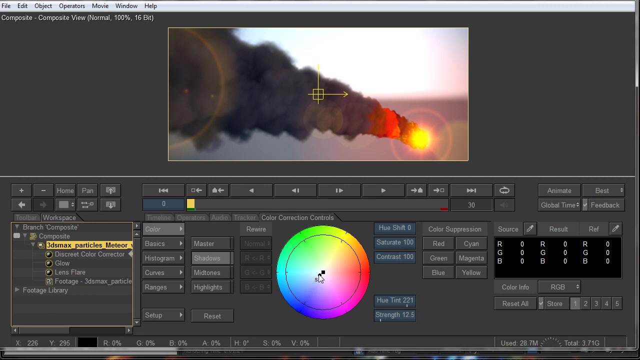 just to have a little bit. let's say that we like to have another luminance to peak, just there, and let's play a little bit with a color correction. I'm trying to find a good look for the image, something like that, and let's go to play a little bit. 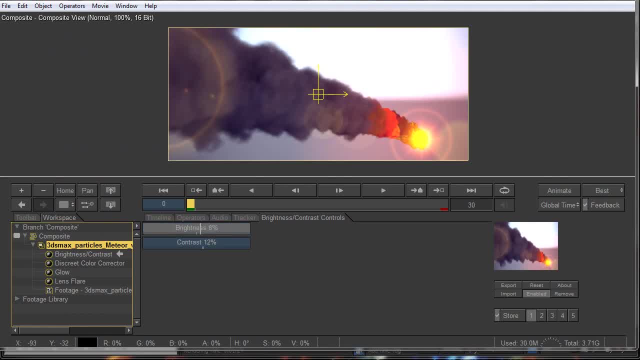 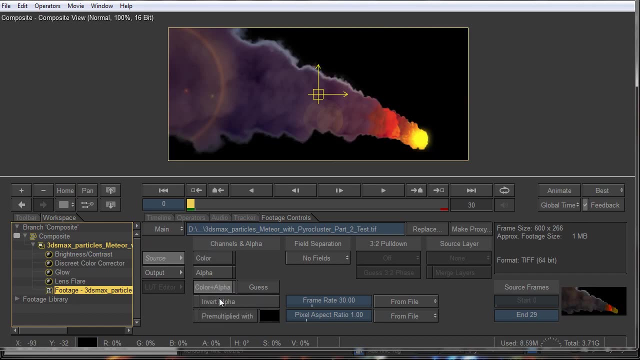 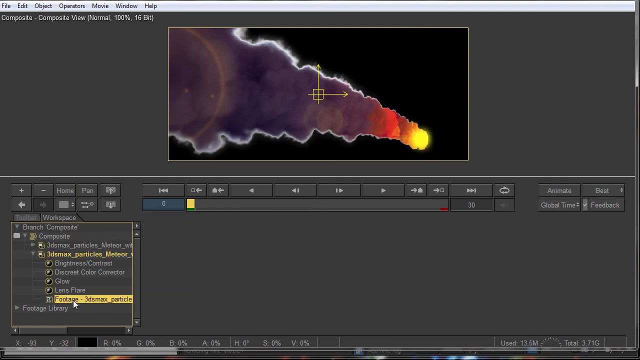 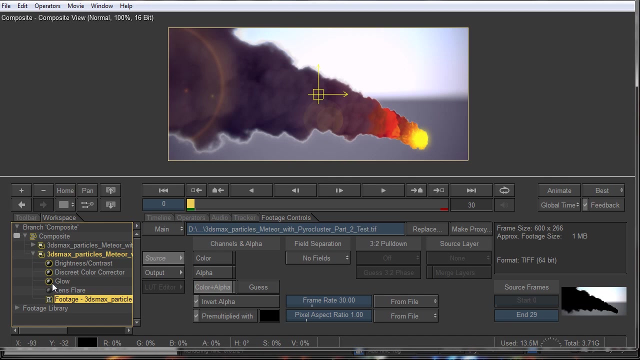 with the brightness and contrast too. I'd like just to see something: ok, so we can remove there the lens flare, the discrete color, best of all, just the discrete color there. let's remove the pre-multiply so we can have a different coloring, brightness and contrast between. 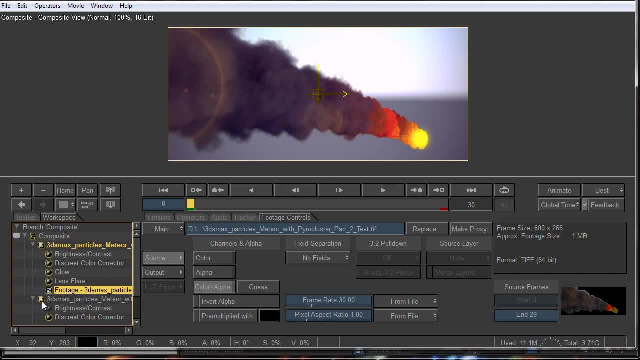 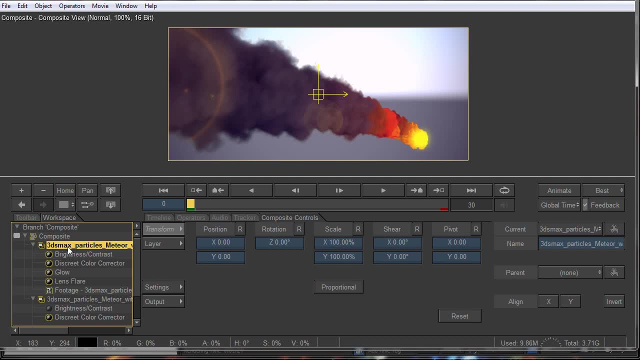 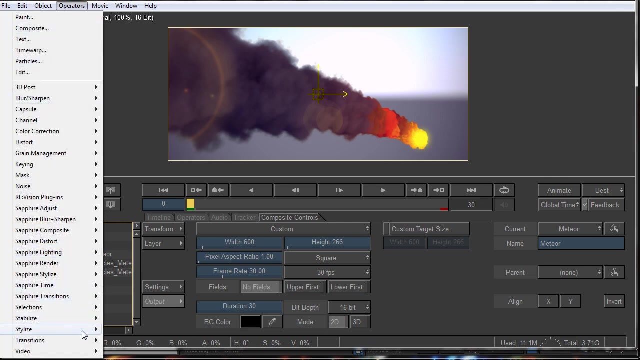 the two stuffs there. so you see, we have the sky on a separate path and in this way there we can have another layer of glow, so we can have both as nesting. let's call it Meteor, and there we say 16 bits and we can have again. 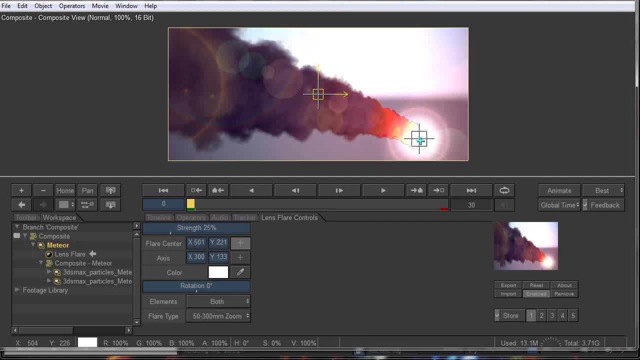 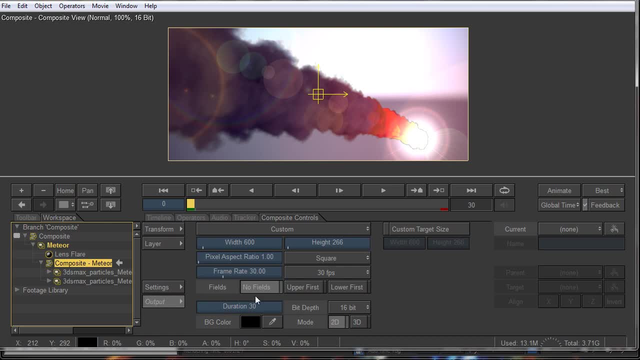 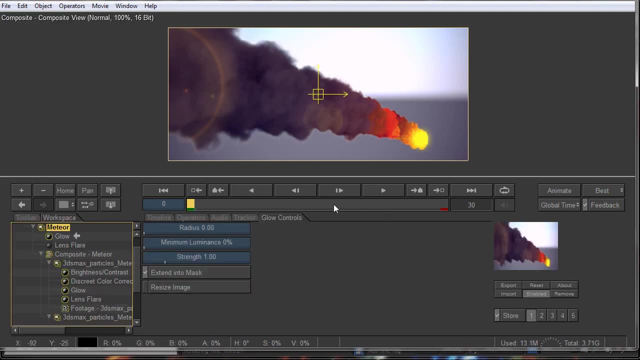 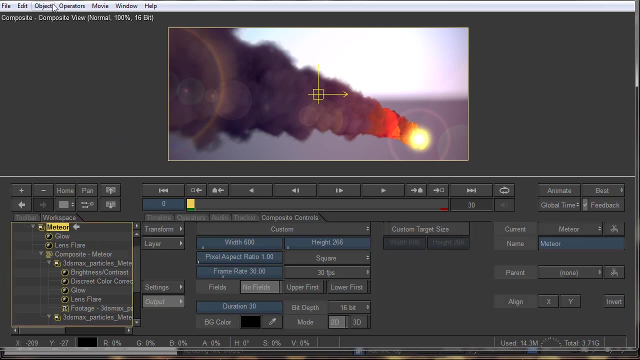 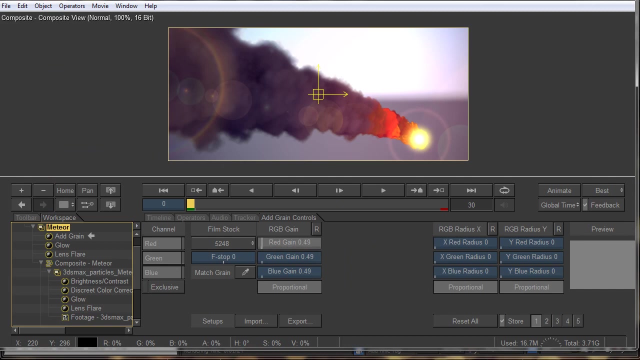 a lens flare before I like to add a little bit more glow. ok, and again, we can have the lens flare there, not just so big, something like that, and we have to move it there, and then we can add a little bit of grain with the needs. 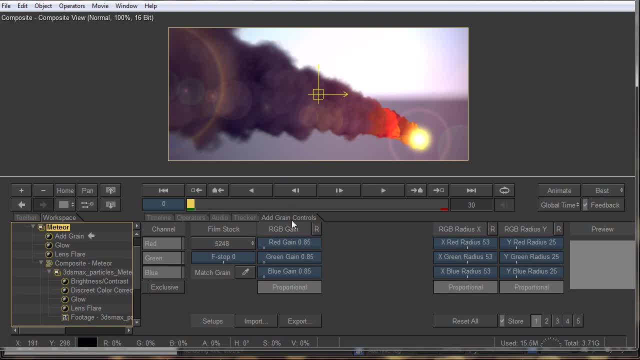 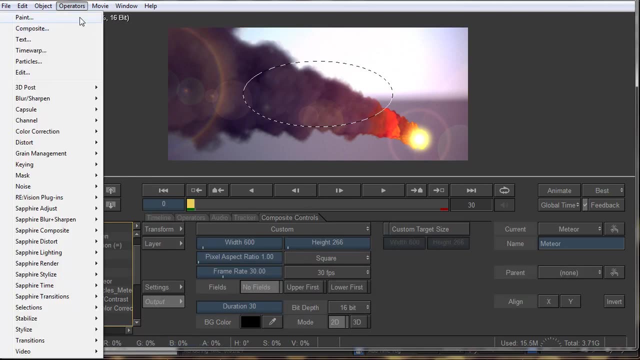 we don't need to play too much with the grain is just to have it inside the scene. so you can leave some parameters really simple and I like to make a selection. so selection, elliptical selection, and we'll try to simulate the vignetting more, more visible.